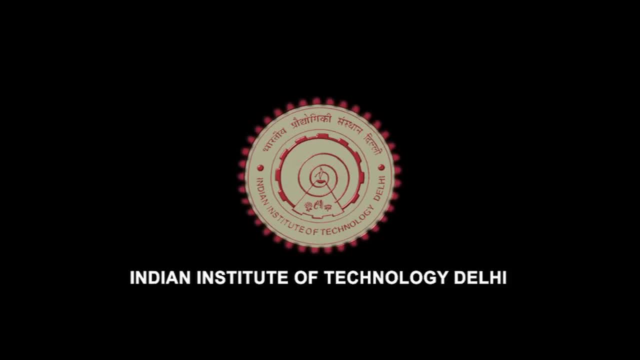 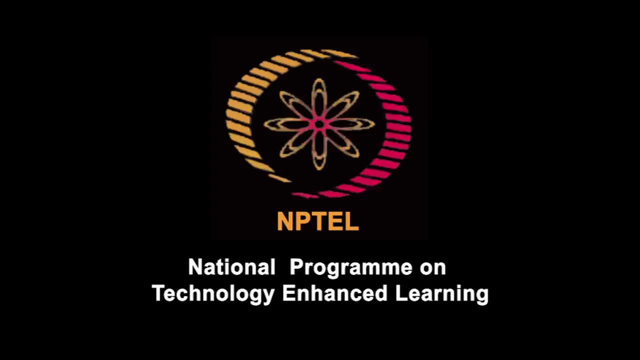 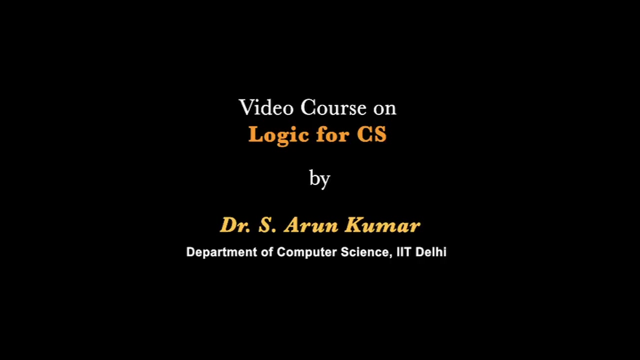 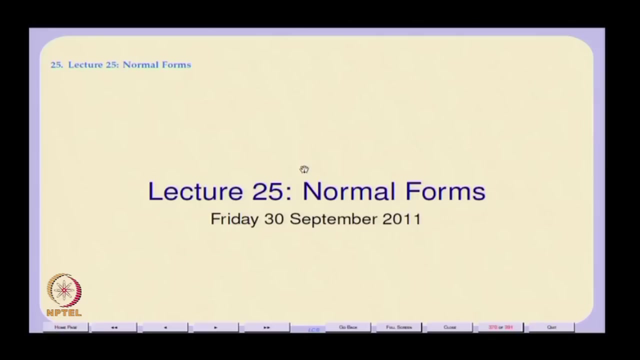 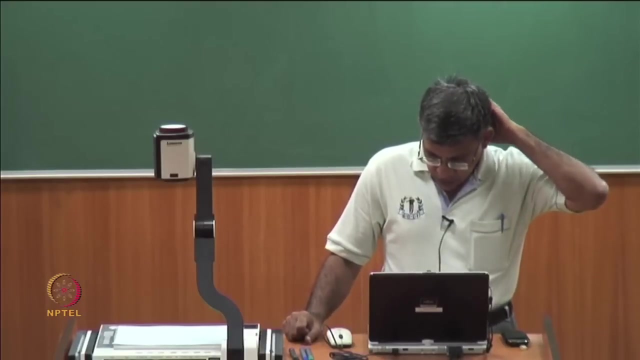 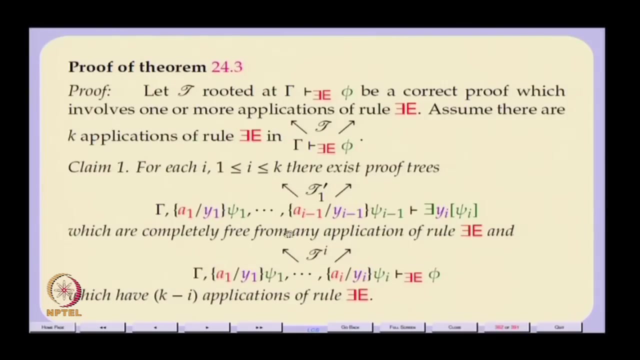 So last time we were looking at this existential elimination elimination theorem. So I have sort of change the proof a bit. There was some bugs that I realized in my original version. They are very subtle bugs but essentially the proof in its essence was correct, but so but. 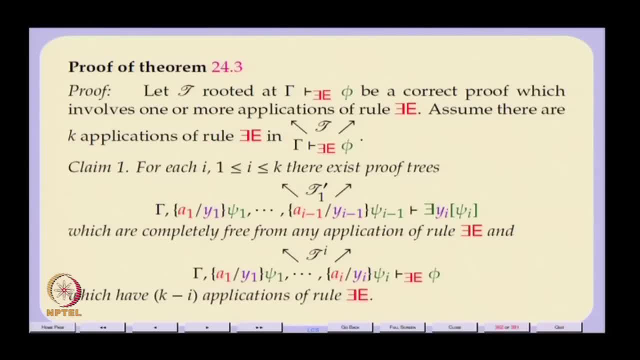 the whole point is this: In you start with a proof tree which uses there exists elimination, and let us assume that there are some k applications of there exists elimination, Then these k applications need not be on the in the leaves of the proof tree. that is the first thing. 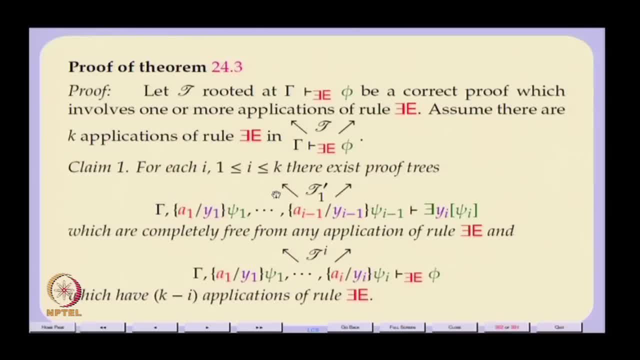 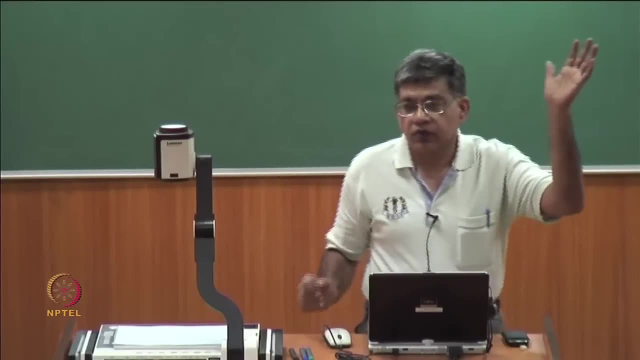 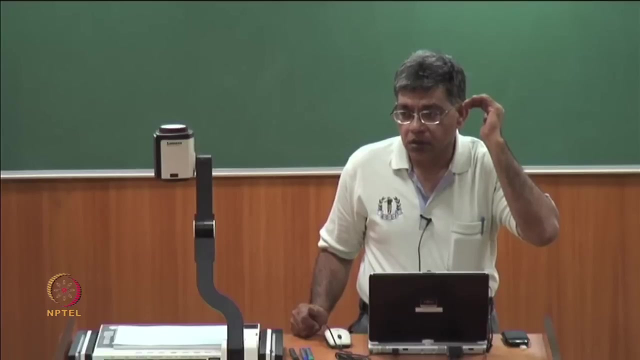 So what you need to do is you need to identify the identify an order of the applications based on the level in the proof tree, So that the you start off by eliminating the ones closest to the leaves and, once you start, eliminated all those ones that are closest. 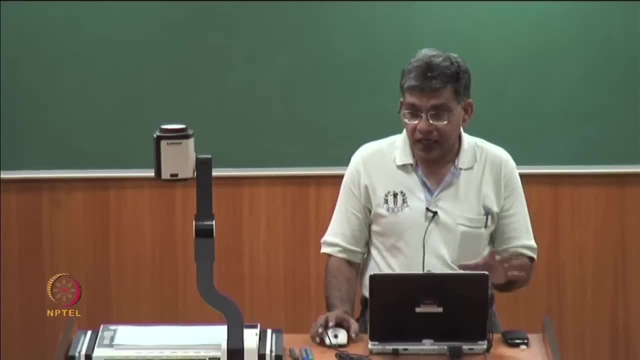 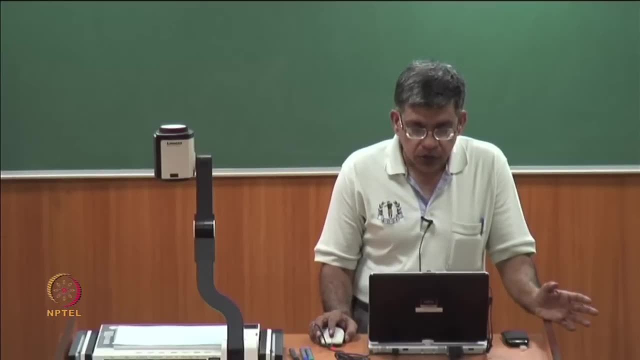 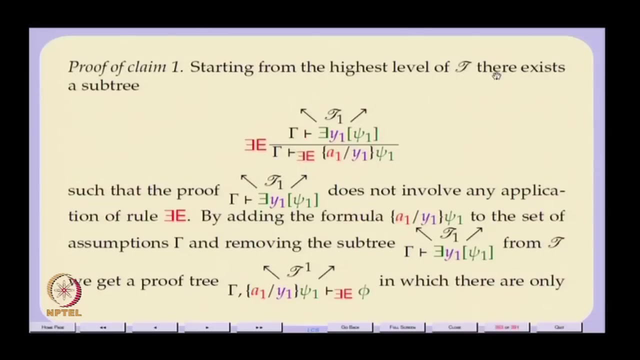 to the leaves, you essentially you get different proof trees because you will now add those things as assumptions. So essentially what we are saying is you start from the highest level of the tree and there is some first application of there exists elimination. So you let us say that is sub tree t 1, which, and if it is an application, 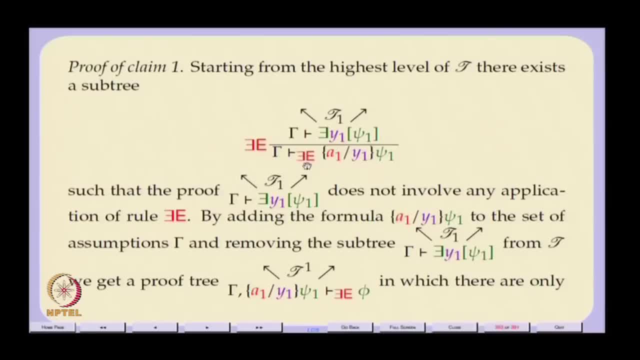 inequalities, there exists elimination than it is a sub tree t 1 root at formula, like there exists y 1, psi 1.. And because of which, when you apply, there exists elimination, you got this first constant, a 1.. Now it is clear this tree t 1 does not have any application. 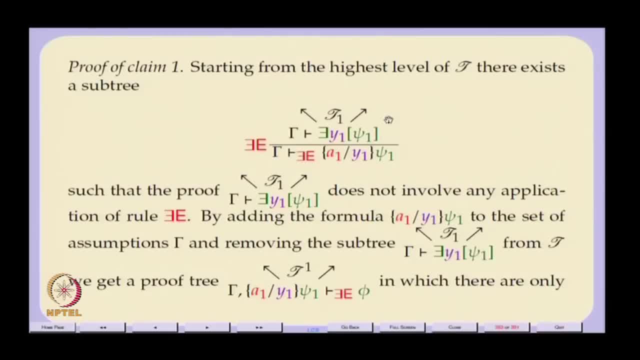 of. So now, when you add a 1 for y 1 psi 1 to the set of assumptions, you remove this entire tree t 1.. But you retain this, essentially this node, with the assumption that a 1 for y 1 psi 1 is an extra assumption. So then that: 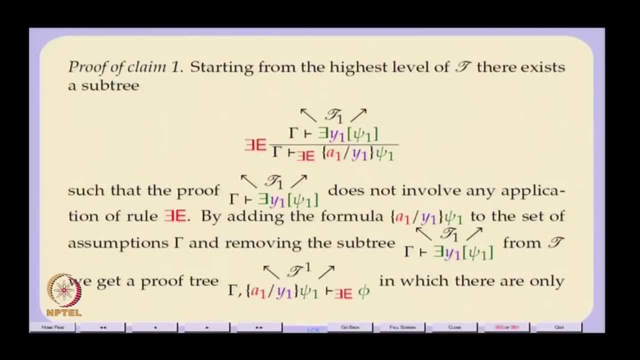 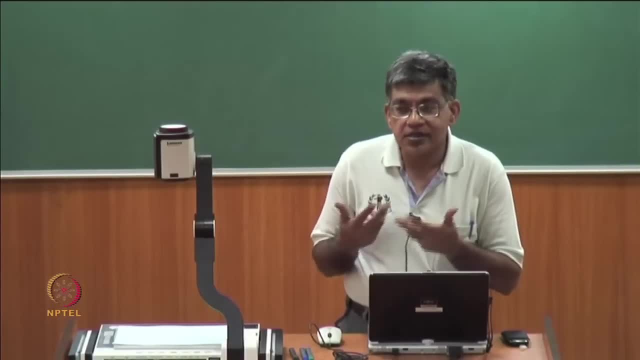 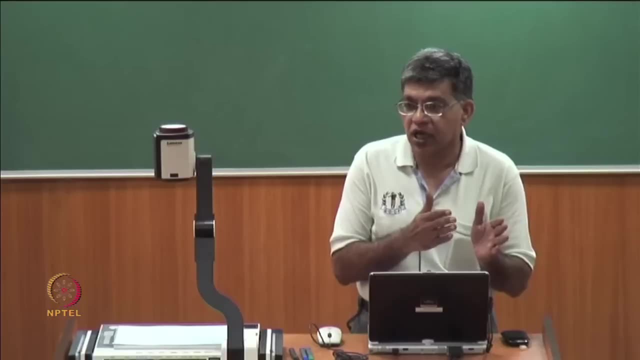 becomes a leaf of essentially a modified tree. Then on this modified tree you look for essentially the second highest occurrence of their exist elimination and remove it, replace it and add this, an extra assumption: a 2 for y, 2 psi 1.. Then look at the modified tree. 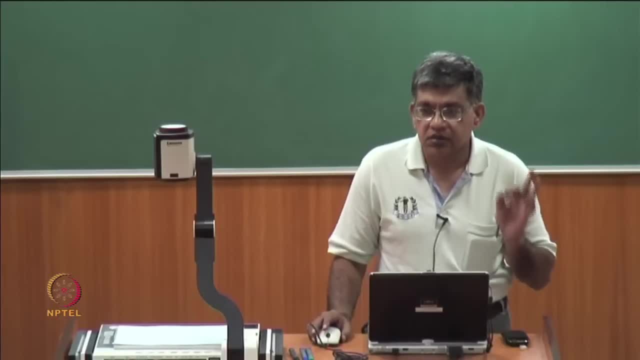 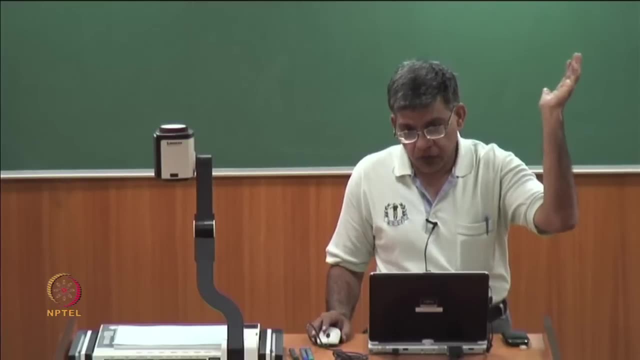 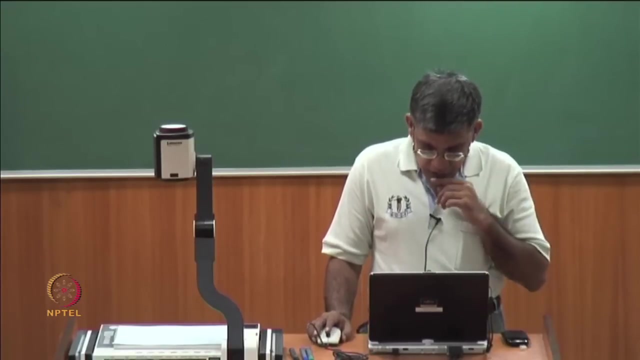 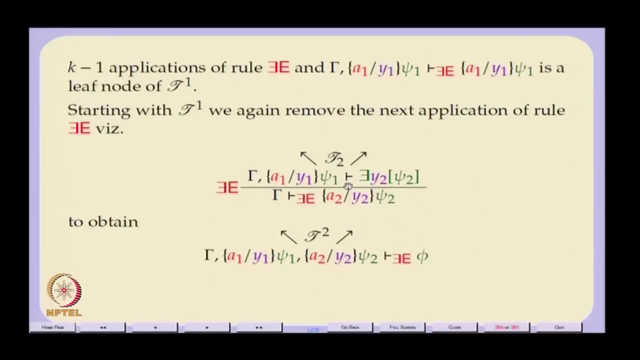 and then look at the highest, and so on. So there is an order, which there is a total order which you can impose, starting based on the levels, starting from the leaves and proceeding towards the root of the tree. So each of this trees t 1, t 2, each tree t i that you eliminate actually is of a modified 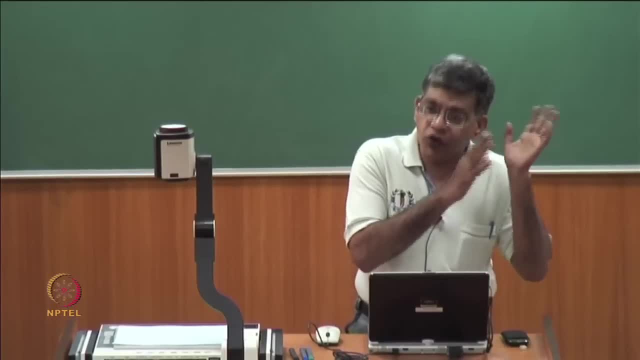 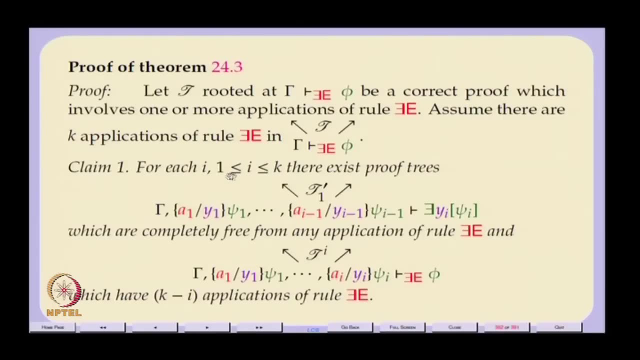 tree of the original proof. So this claim here essentially says that for each i one there are k applications of the rule in the original proof. for each i proof trees t 1 prime. this should be t i prime gamma, with constants a 1 to a i minus 1 replacing. 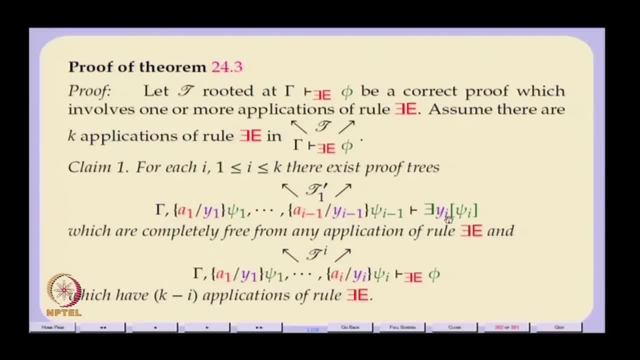 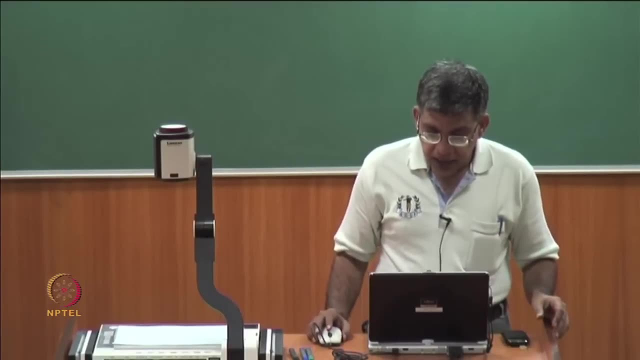 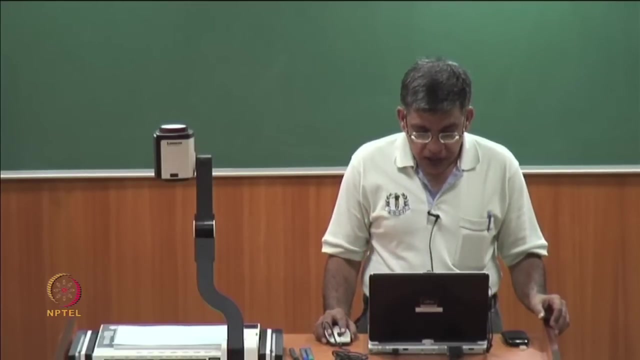 y 1 to y i minus 1 proves there exists y i, psi i, and this proof tree does not have any application of there exists elimination, And the act of removing these sub trees and therefore getting modified proof trees means that. so these, all these proof trees, t i primes. 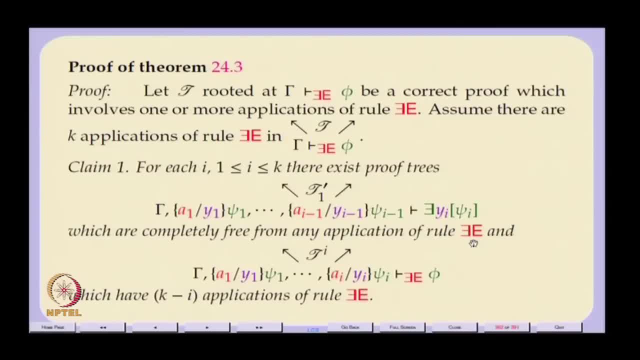 are completely free from any application of the root. there exists elimination And the modified original proof tree. with each modification at the ith stage you get a proof tree, t, i, t, superscript, i, which has these i as some i extra assumptions and which proves phi And of course, there are k minus i applications of there. 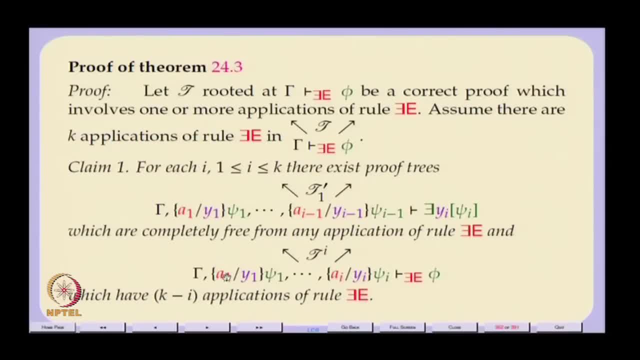 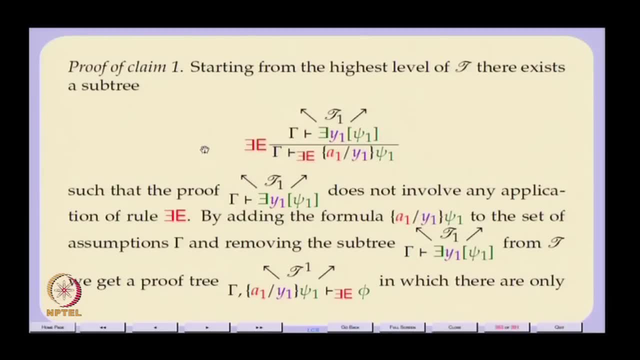 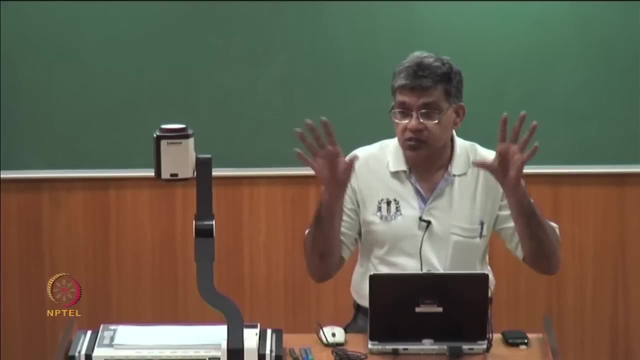 exists elimination in this proof tree. right, that is so. this claim is so. this claim is important in my in my original proof the other day i So i actually assumed that all these application could be taken as per the leads, But that is not true, because if i had existential quantifiers deeply nested inside the law, 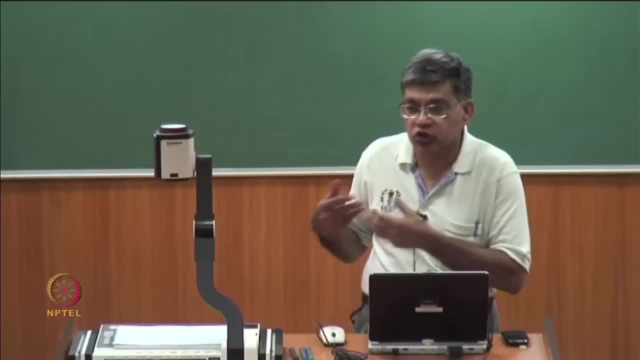 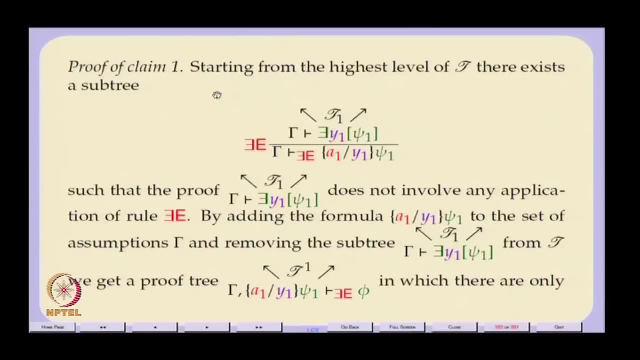 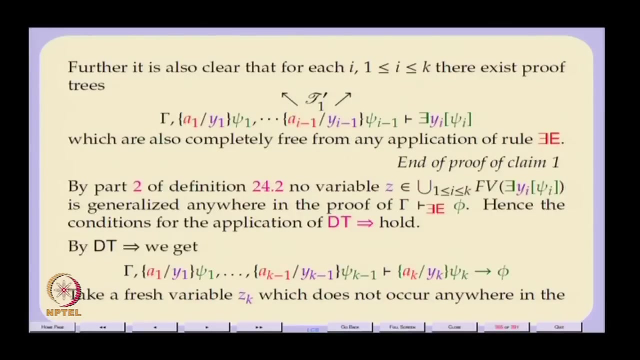 formula a, then i will have a extract out all the root nodes and go through several steps before i before i eliminate them. So this is the modification. So essentially this claim can be proven and it goes into several. so there it ends and 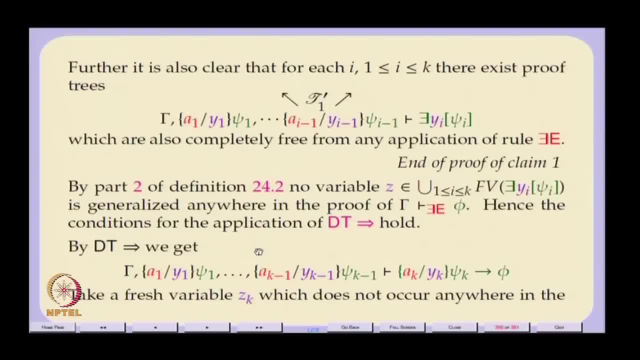 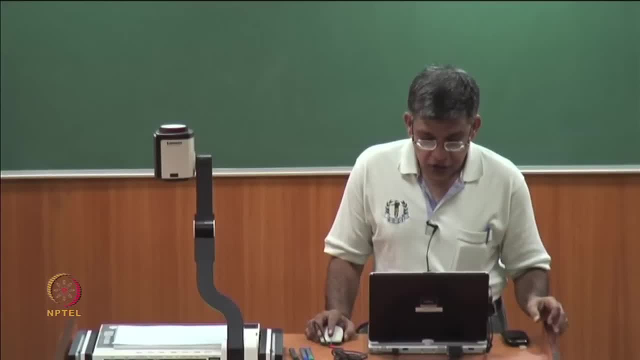 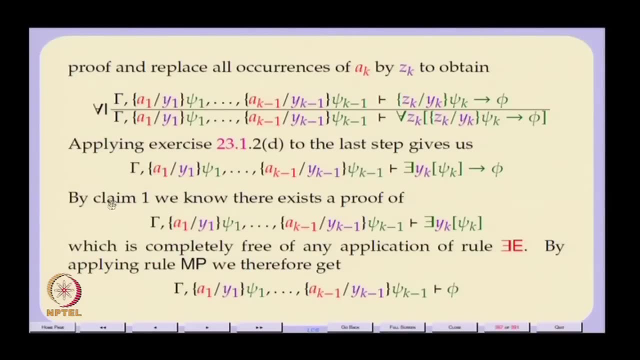 after that. essentially we use the fact that each of those t? i's did not use their exists elimination in order to apply this modus ponens. So here I had written something which was wrong. So by claim 1 we know that there exists a proof of this. a 1 to a k minus 1 psi k minus. 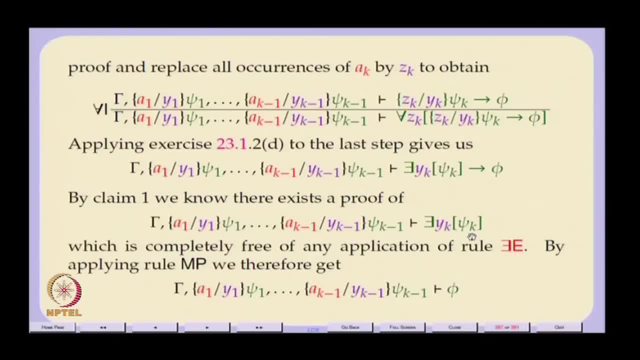 1 proves there exists y, k, psi, k. We know that there is a proof of this which is completely free of any application of this rule, And you also have obtained, through the last step and reduction theorem. you have obtained this and therefore you can. 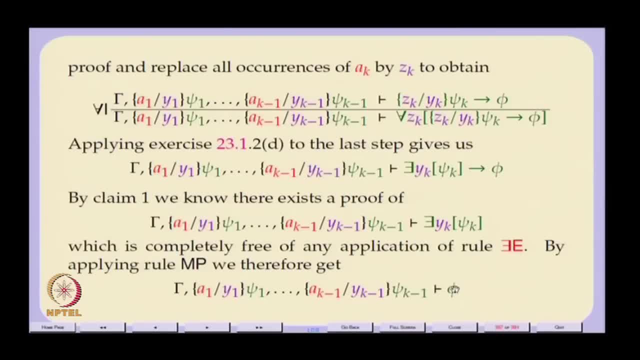 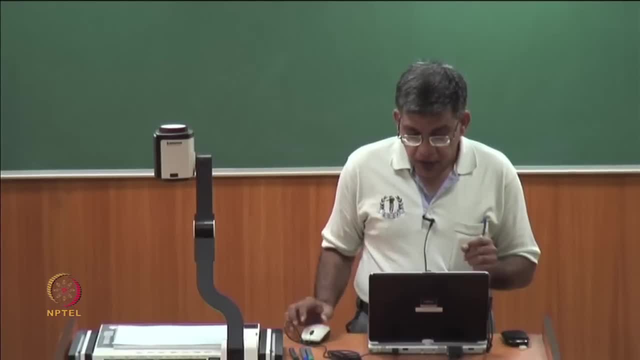 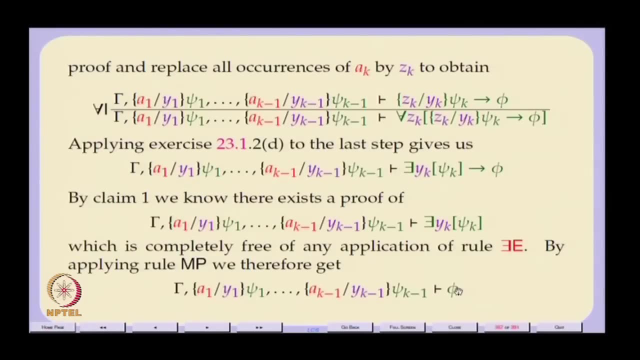 Now apply the rule m p and you can get this, get this result. and now, with this new tree proof tree, Now this proof tree, you can now start eliminating a k minus 1 and you will get a new proof tree, and so on and so forth till you have eliminated all of them. 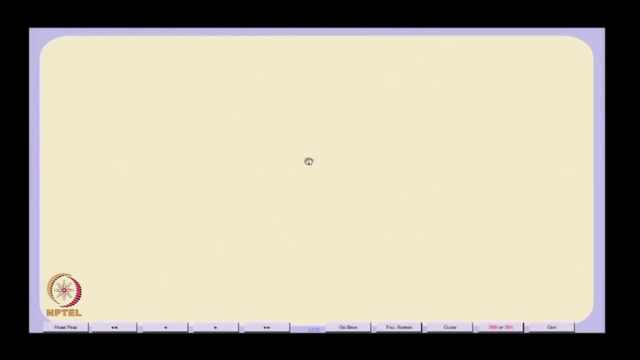 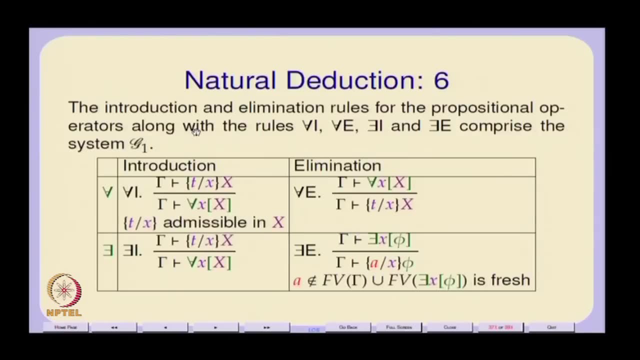 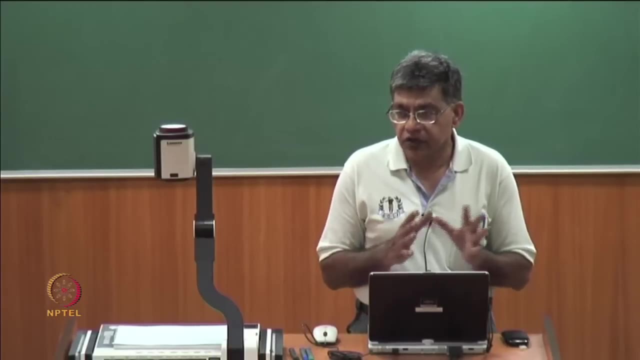 So this is. by the way, I have also added a large number of exercises which you should look at. Some of them you may have to submit. So now, what it means is that? so there are. So we have got existential elimination and we have got existential introduction. So essentially, 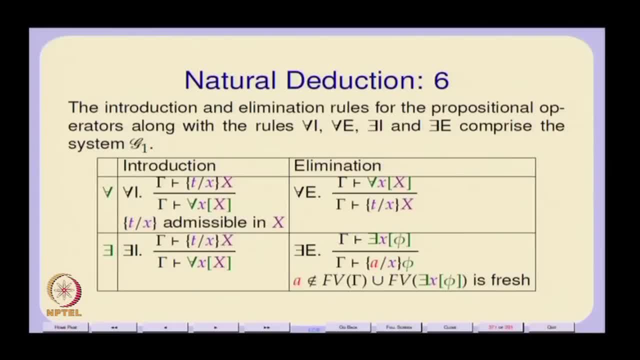 what we have is a full natural deduction proof system. that is it. There ends the matter as far as natural deduction is concerned. there ends the matter. So, for all introduction- and there exists introduction and elimination rules- and add it to those propositional introduction and elimination rules and you have a complete 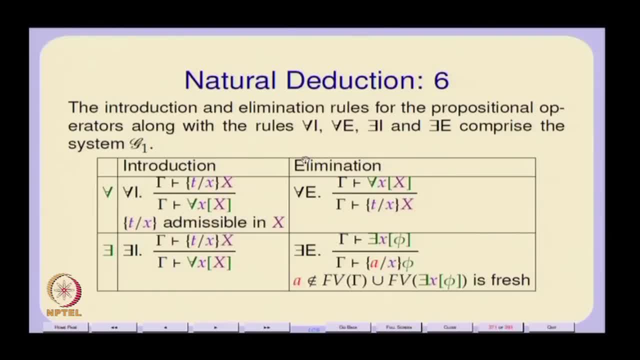 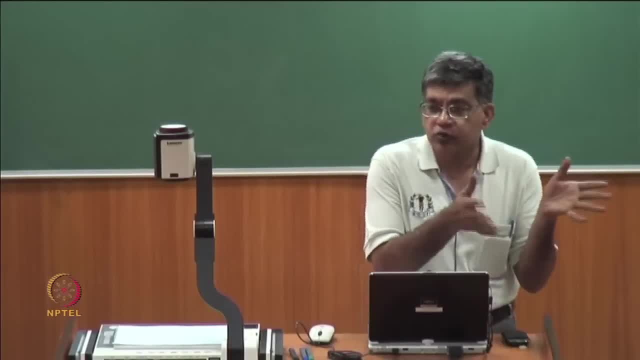 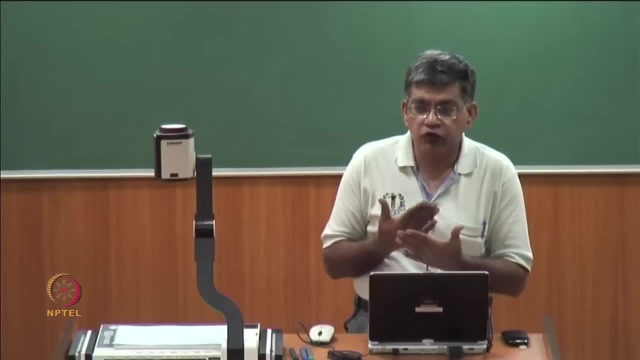 natural deduction system, Except that the proofs in natural deduction now, because of there exists elimination, will look different from the proofs of the Hilbert's size system, Whereas in the propositional case you could actually prove every rule of the natural deduction. 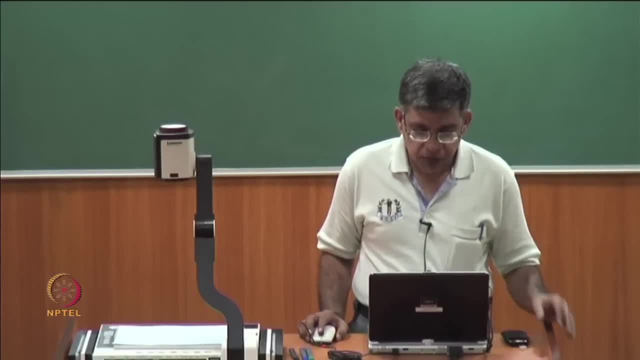 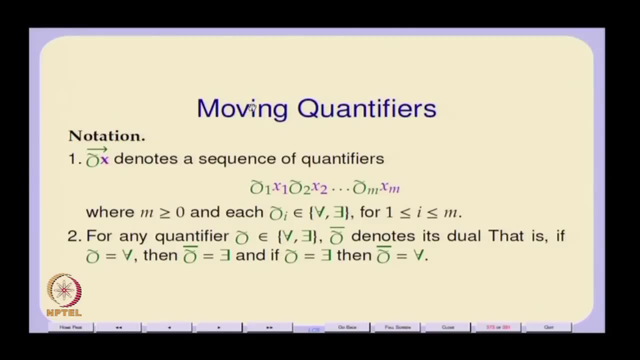 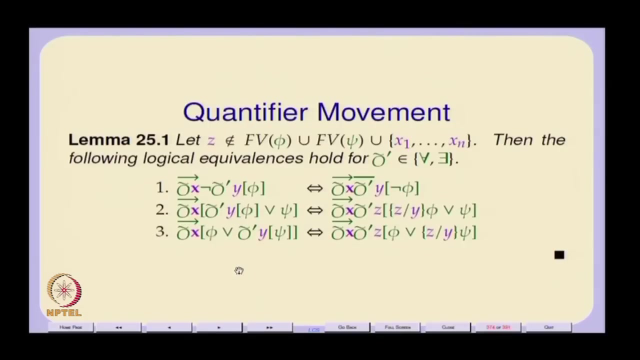 So there are a lot of this is all for you to have fun. So now let us get on to essentially the main thing now of moving quantifiers. So I am going to introduce some heavy notation, So I am going to introduce equivalences, which is homework for you to prove Notice. 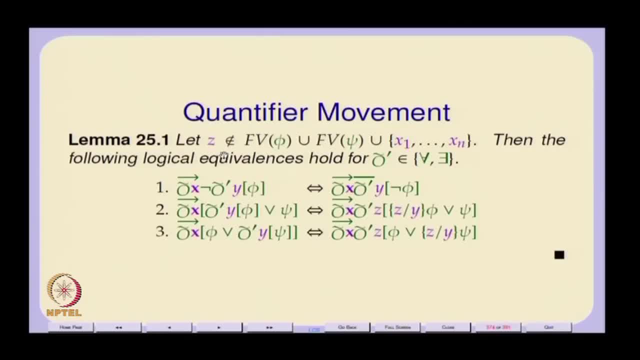 that there are some conditions you have to fulfill. these equivalences have to fulfill. Firstly, I am assuming that there is a variable z which is not free anywhere in any of these and it is not any of these variables which are essentially going to be bound Then for 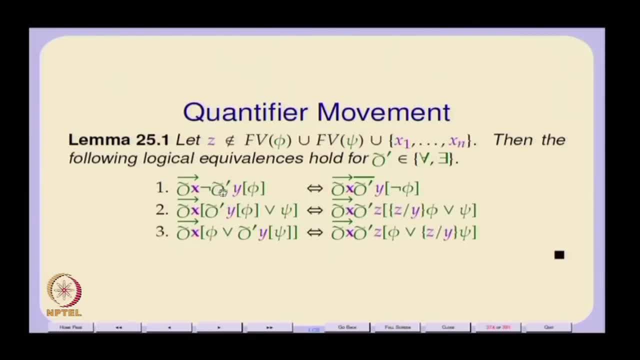 any vector of quantifiers followed by a, not q, prime. where q prime is one of the quantifiers, Of course this is just like your De Morgan's law. then you invert the quantifier q prime, So you get q prime bar and you negate the body of this thing And here you have q prime. 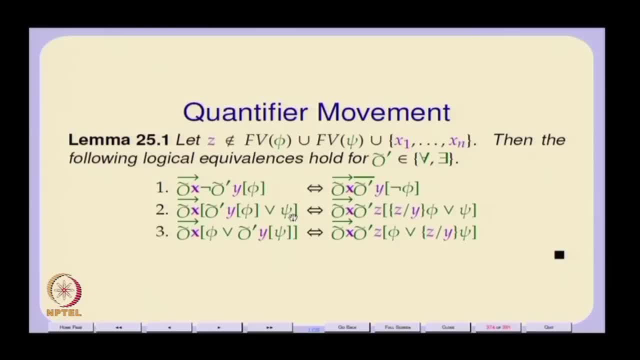 y, phi or psi. So what I am going to do is I can do an alpha conversion and replace that y by a z, and since z does not occur anywhere in all this, I can also move this quantifier prime z outside. So this is, and this is for r, and similarly, if the quantifier occurs on 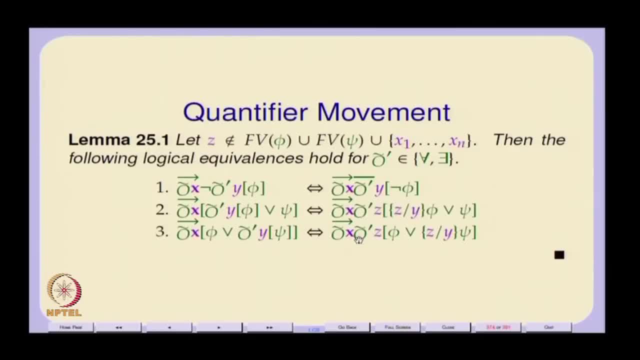 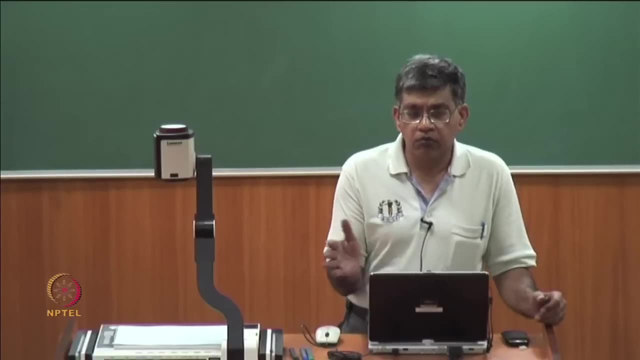 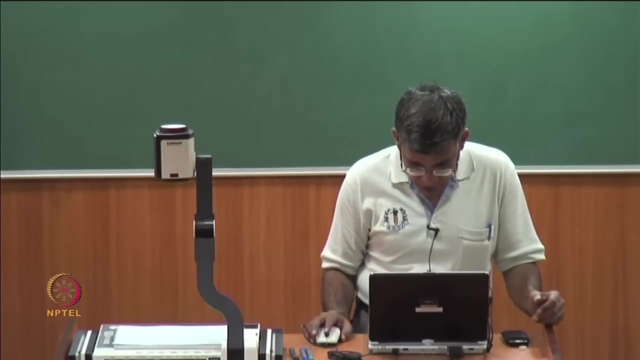 this side, then I can rename it and move this quantifier outside. So look at these, look at these logical equivalences as operating from left to right. So what, you? what are we doing? moving quantifiers towards the left, of the right, yeah, of a any term. 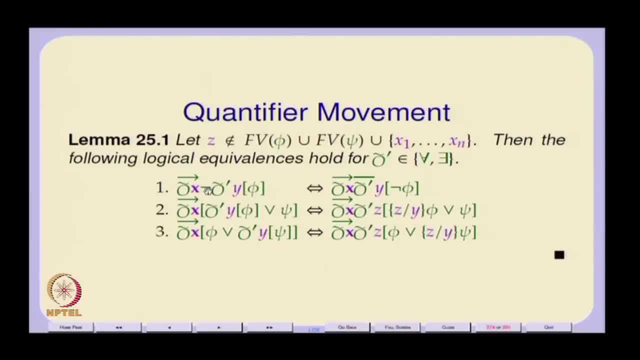 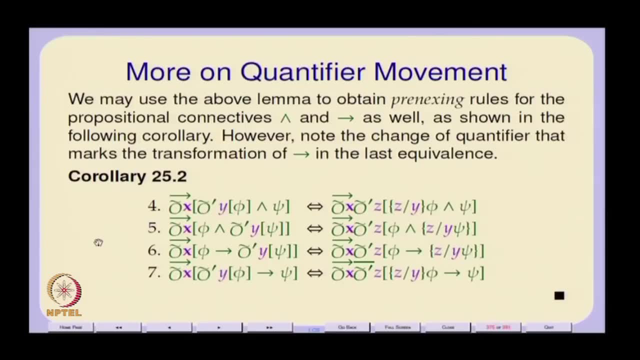 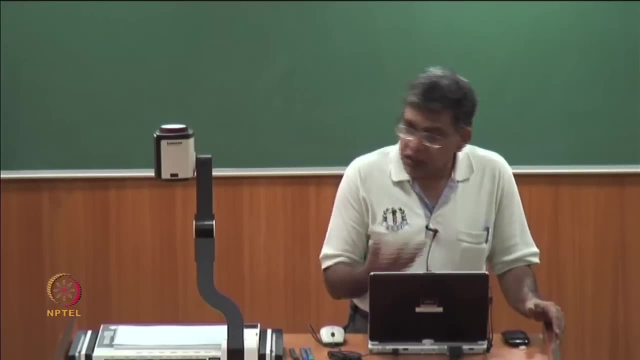 this for not and or. it follows as a corollary that you can do similar things for the other operators. So now- I mean now that we have got our natural reduction system and so on- we can consider the full language, and so we will work with. 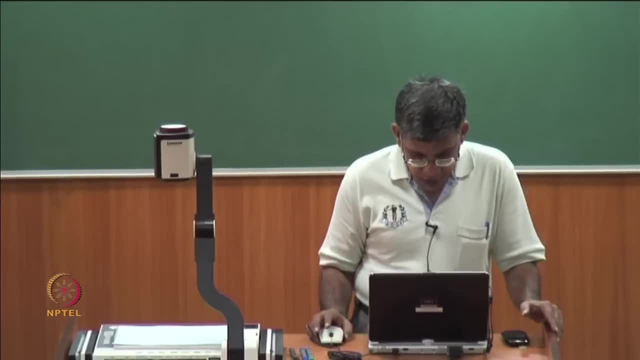 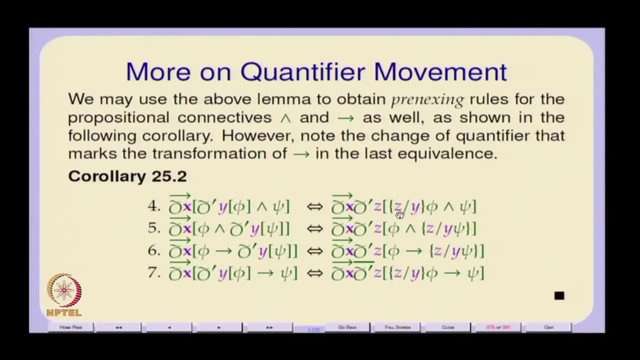 the full language that is. So here you have for, and if you have q prime y, then I replace alpha. convert that q prime y phi to q prime z, z for y in phi, and since z is new, I can move this quantifier out. And similarly in this, in the case of these arrow, of course. 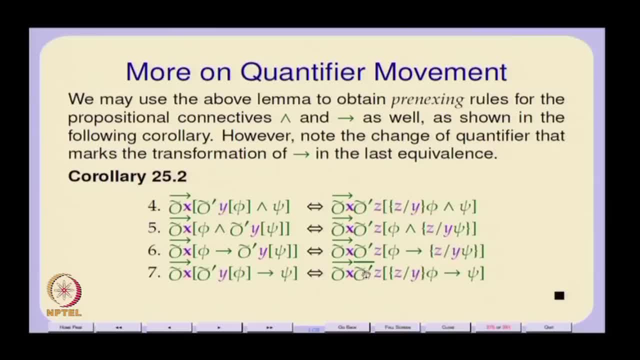 in arrow. it includes that particular thing, right. there is this inversion of the quantifier in the last, which we have already seen, we used it in in our proof Of there exists elimination elimination theorem, right? So this is the last one which corresponds to that and actually it works for both quantifiers. the inversion of the 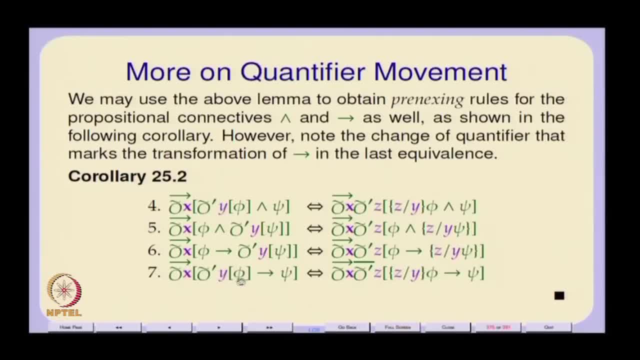 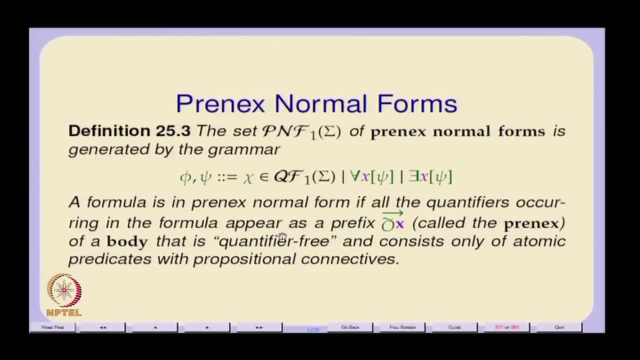 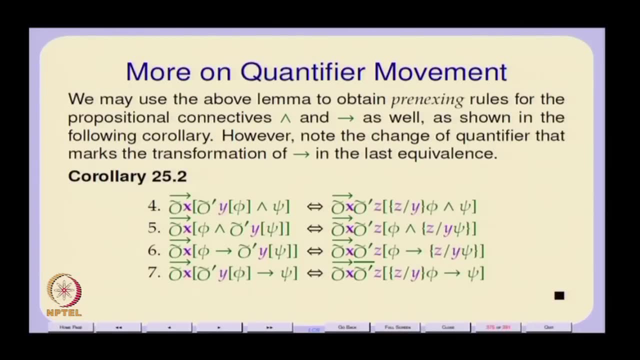 quantifier happens for both quantifiers, and that is what this is supposed to. once you have this, if you look at these 7 rules from left to right, that left hand side being, In this case, by the right hand side- then what happens in each case is that quantifiers are. 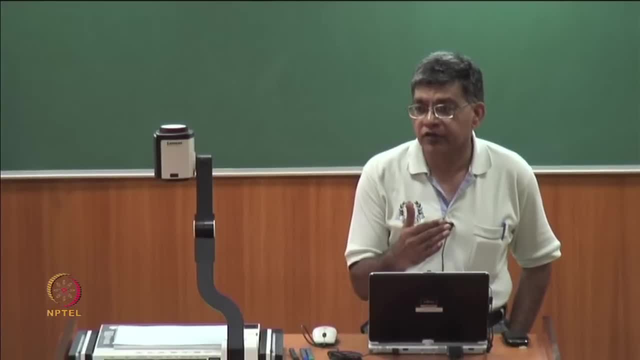 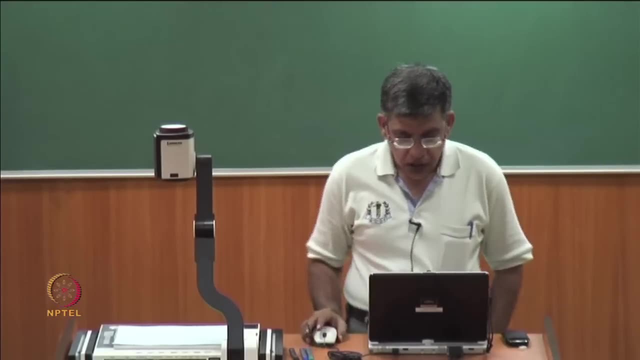 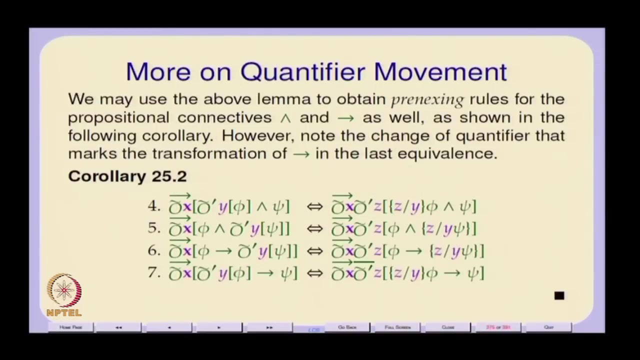 being moved from inside to the outer levels of the abstract syntax tree. I mean, they are being moved closer to the root of the syntax tree, right? So these 7, these 7 logical equivalences essentially take care of negation and or and arrow. there is no. 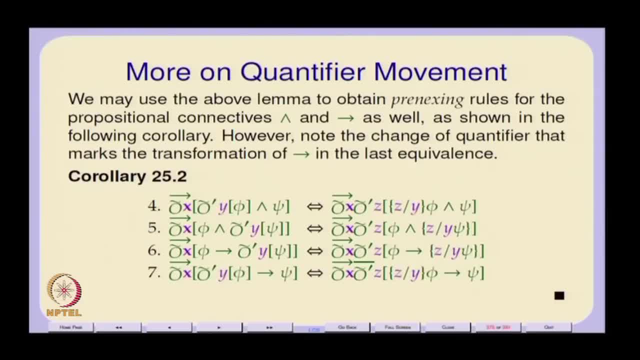 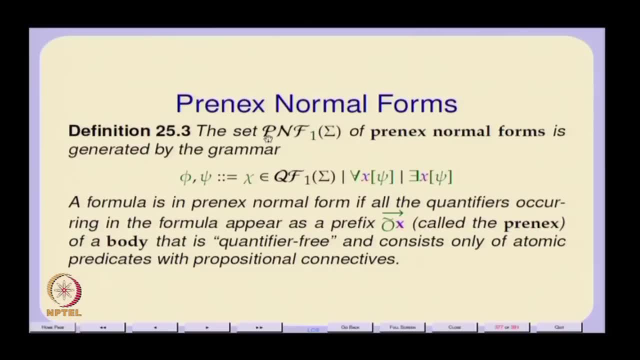 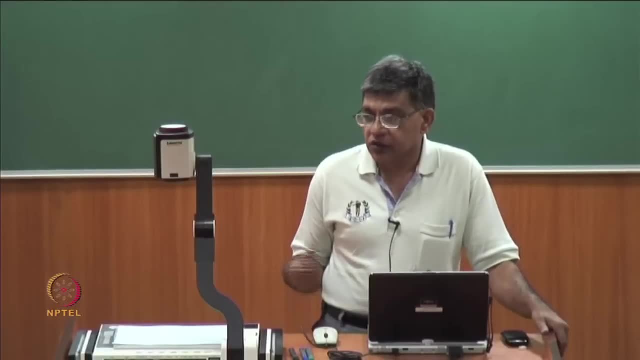 Similar logical equivalence for the by conditional, or no obvious logical equivalence for by conditional anyway. So what this means is that now we can define a sub language of the full language of first order predicate logic called the set of green x normal forms. So 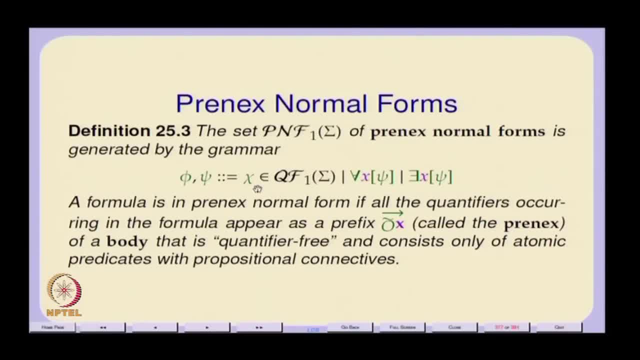 this is so. you take any quantifier free formula in, So in the quantifier free subset of first order logic, so that is chi belonging to q, f, 1 of sigma, and then you can keep adding quantifiers to the left. So the formulas. 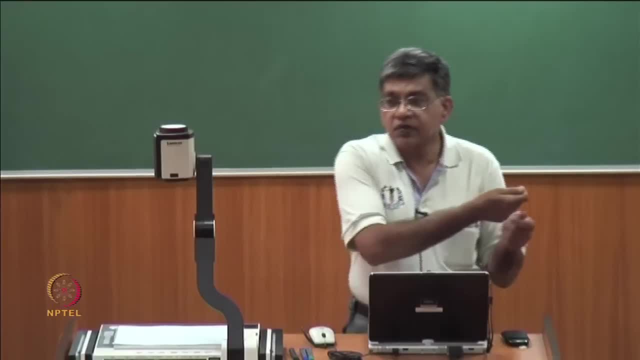 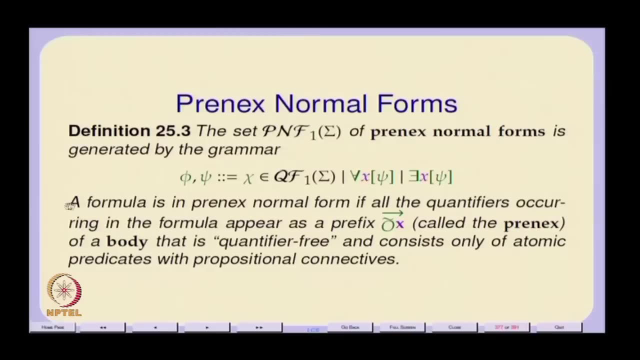 that are generated are such that there is a sequence of quantifiers and then there is a quantifier free body. that is so that is a pre next normal form. So a formula is in pre next normal form if all the quantifiers occurring in the formula appear as a prefix. 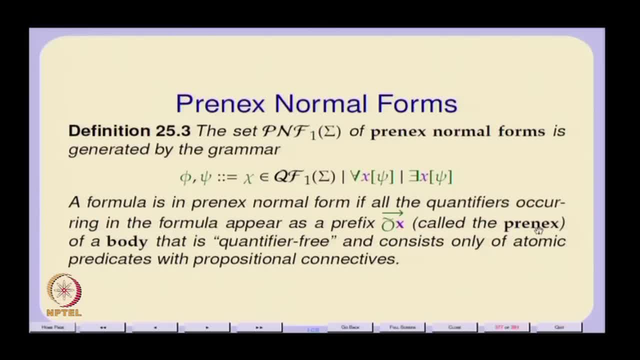 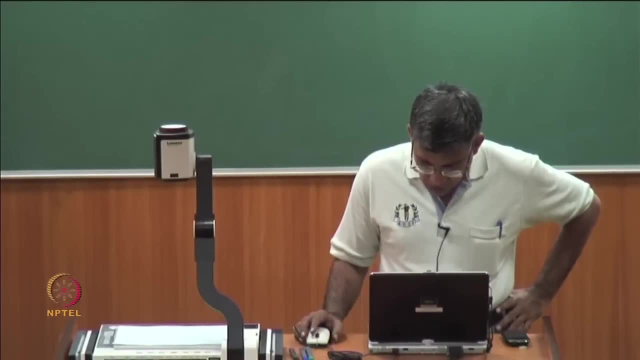 which is a vector of quantifiers which is called the pre next. And then there is a body that is quantifier free and consists of only atomic predicates and the propositional connectives, not or, and and so on. So the pre next normal form theorem says that for any first order logic formula there 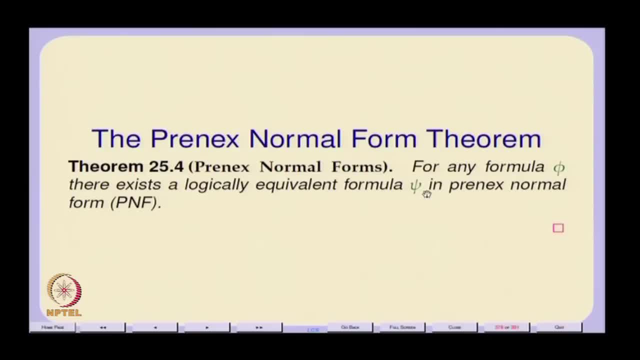 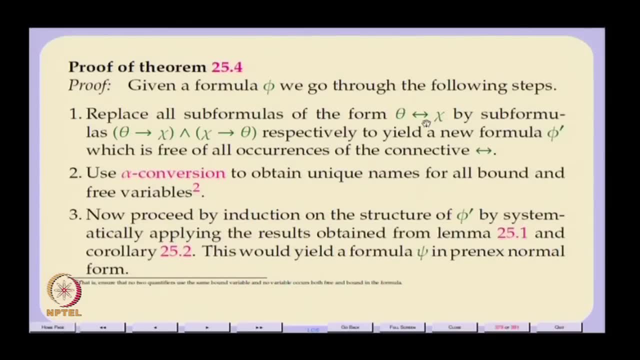 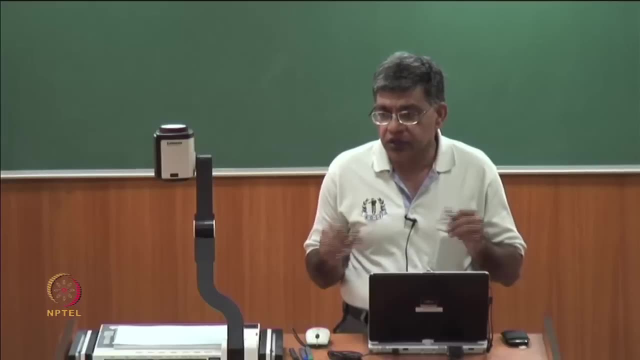 is a logically equivalent, And then prim formula in pre, next normal form. And the justification is essentially just that when I have by conditional, I replace the by conditional by two conditionals, And after that so I replace all by conditionals by the two conditionals given by this And 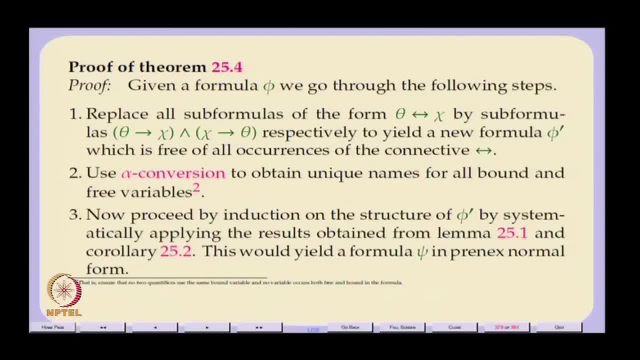 after that, what I do is I use those seven logically equivalency, essentially to move the quantifiers. So, and I basically I use, for one thing is it is, if I am moving quantifiers forming a sequence of quantifiers, I want all the bound variables to be distinct, for example, So, which means that one has to use alpha. 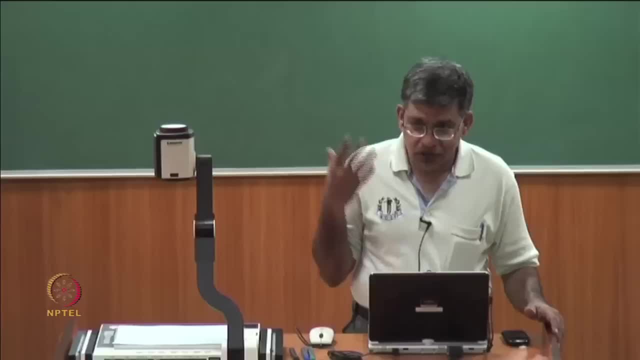 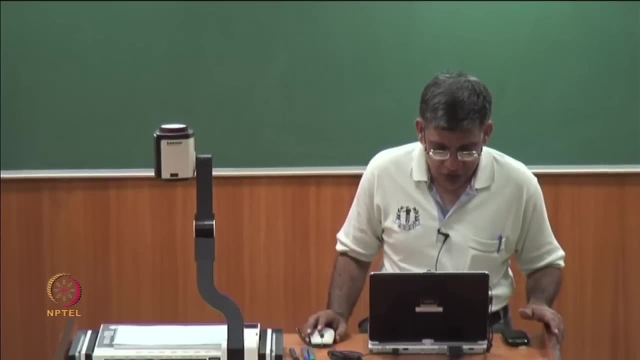 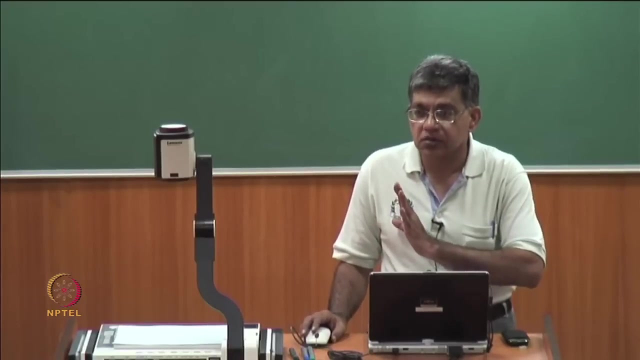 conversion, but now we know that alpha conversion can be done. right to something we took for granted all our lives till we saw the proof of alpha conversion, So that you can get unique names for all bound and free variables. there is absolutely no clash of names. 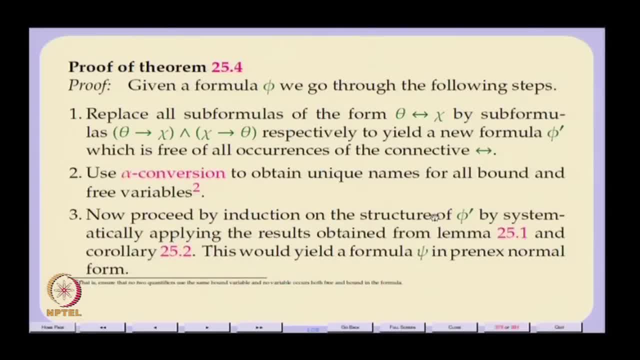 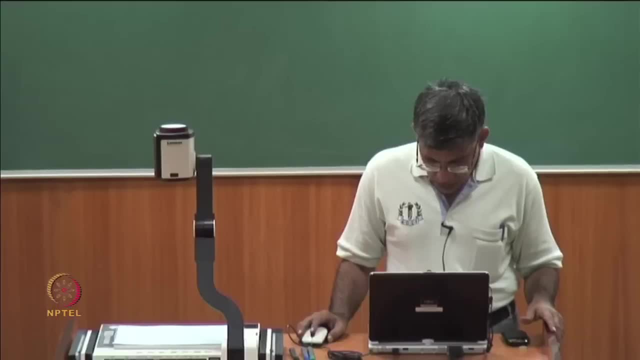 And then what you do is proceed by induction on the structure of that formula to move all the quantifiers by applying appropriate logical equivalences here. So then this would yield a formula psi in prenex, normal form, basically What we also have from propositional. 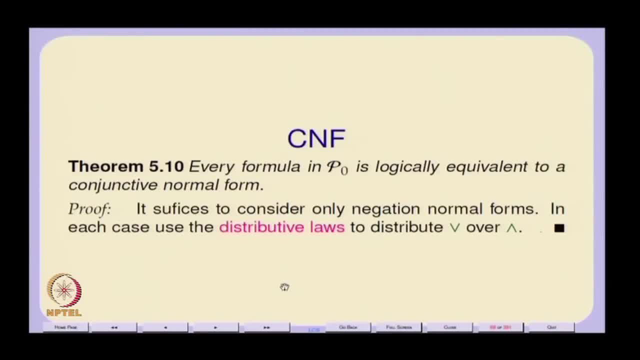 logic is that every formula in propositional logic can be converted into a conjunctive normal form. So basically, one just uses the distributive laws to distribute r over, and one uses negation and so on and so forth. And so now what it means is, since we have a prenex, normal- 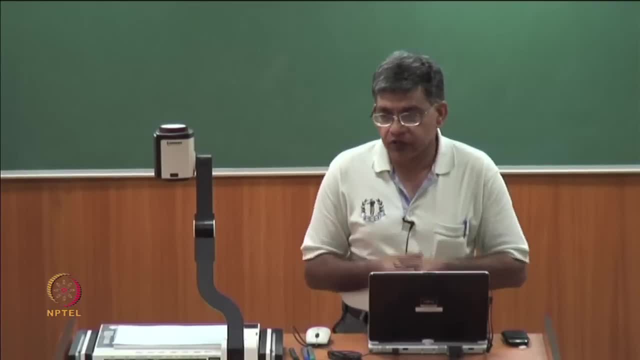 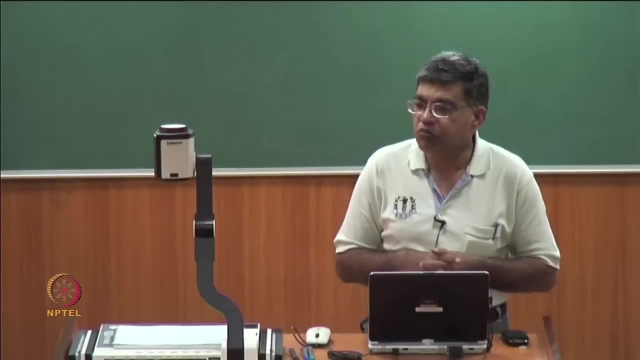 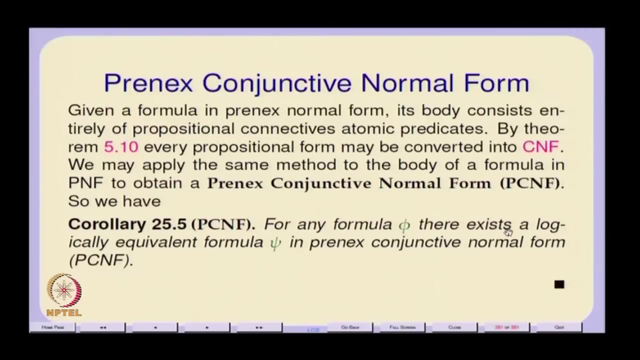 form. we can take the body- the body is just a propositional form- and use the conjunctive normal form algorithm to transform it into a prenex conjunctive normal form. So one obvious corollary is: for any formula of phi there exist a logically equivalent. 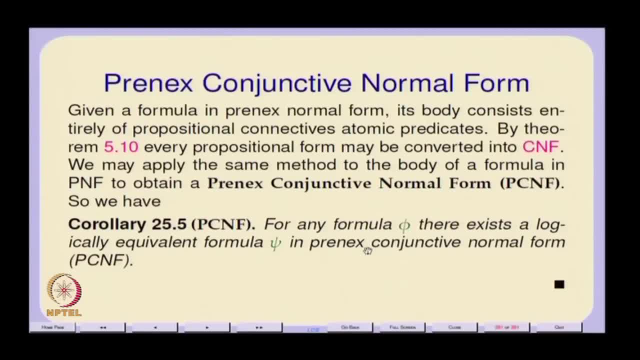 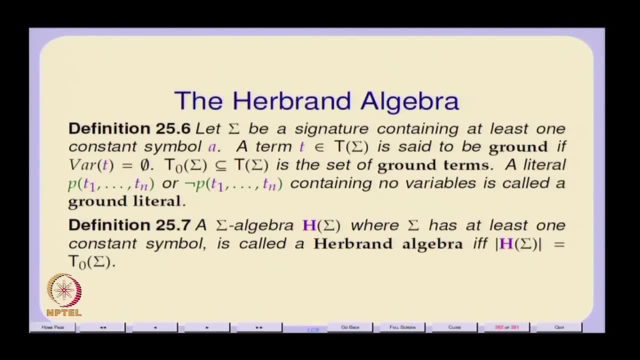 formula of psi in prenex conjunctive normal form. Now we are going into the interface between proof theory and model theory. One of the things that we did was we defined the semantics in terms of certain structures. So let us, Since I do not have any link, I will not go back there. So now what I can also do is: 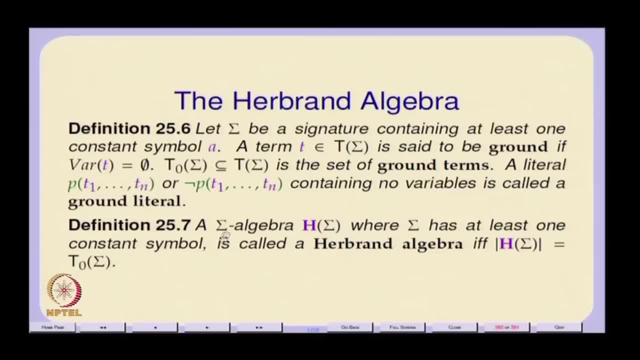 I can for any signature containing at least one constant symbol. Basically this means a function of arity 0. that is all there is to it. A term is said to be ground if it is variable free if there are no variables in the term. So t naught of sigma is the set of ground terms. 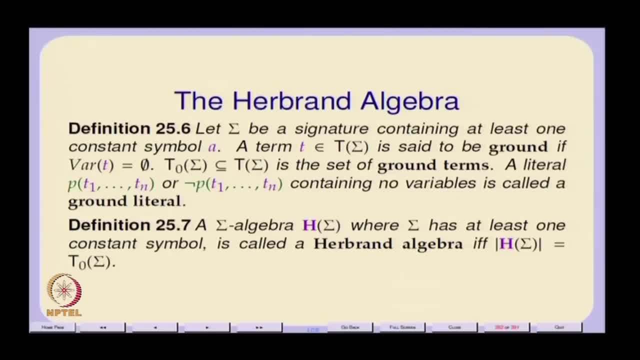 t, sigma is the entire term, algebra I mean, loosely speaking, t, naught and t are all. they are not things in brown, really, they are all things in violet color, that is by my color coding conventions. So a literal is a ground literal if it is an atomic predicate or a negation of an atomic predicate, in which all the parameters 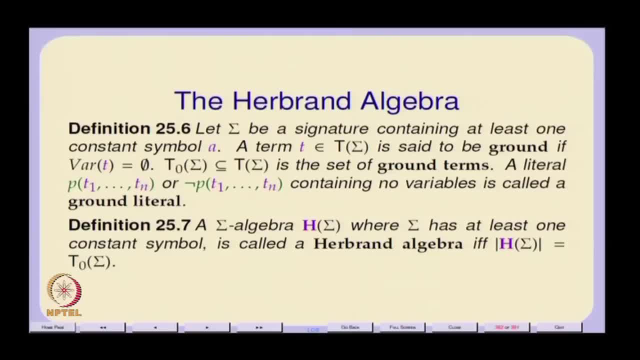 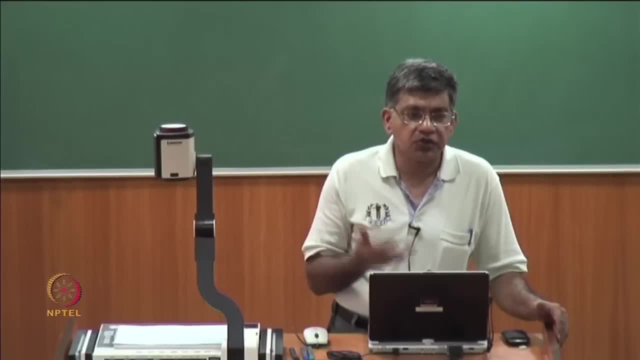 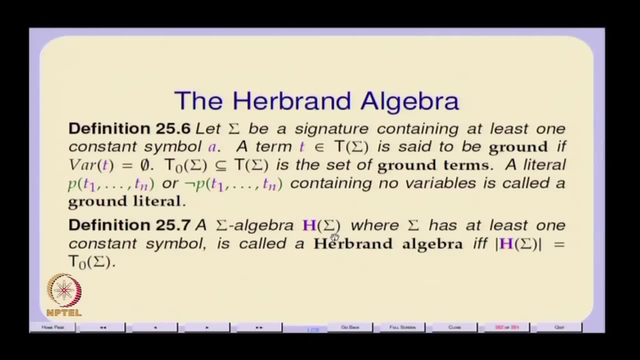 are variable, free. So a literal is. so, as we did in the case of resolution, in proposition logic you have the notion of a positive and a negative literal, And we will. now what we can say is: we can think of this t sigma itself. So 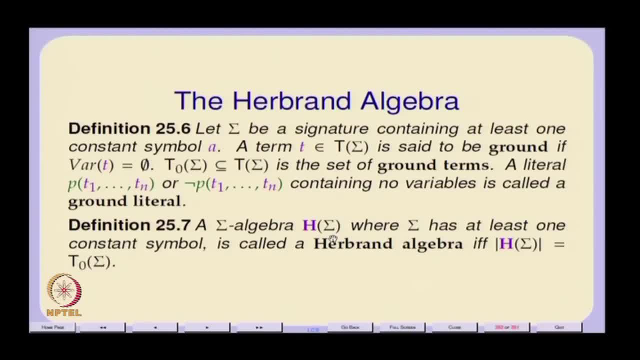 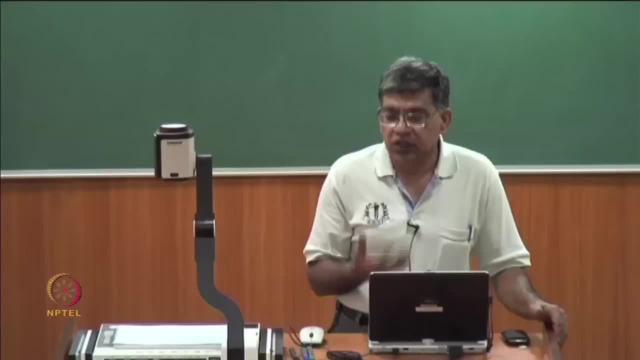 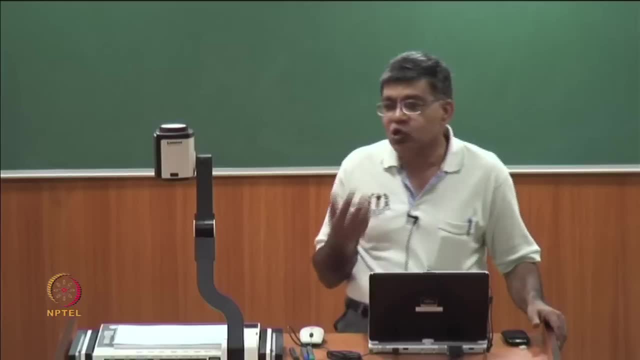 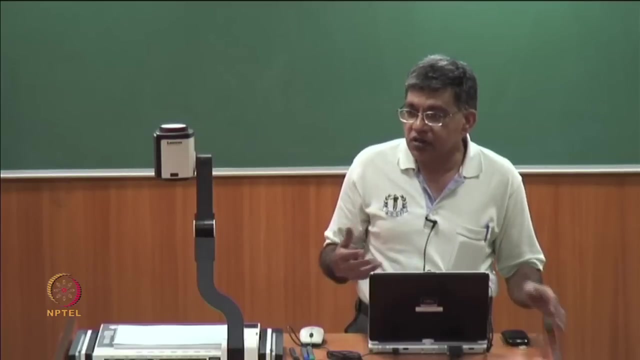 t sigma itself as a carrier of a sigma algebra, So as a domain of a sigma algebra, if t sigma itself is a domain of a sigma algebra, And of course t sigma is closed under the functions of sigma, under the all the operations in sigma. So therefore t sigma is an actual carrier. 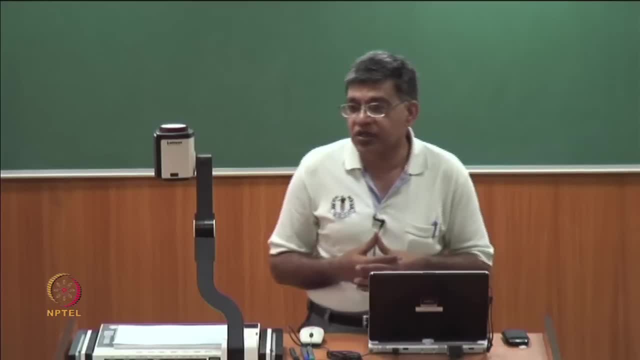 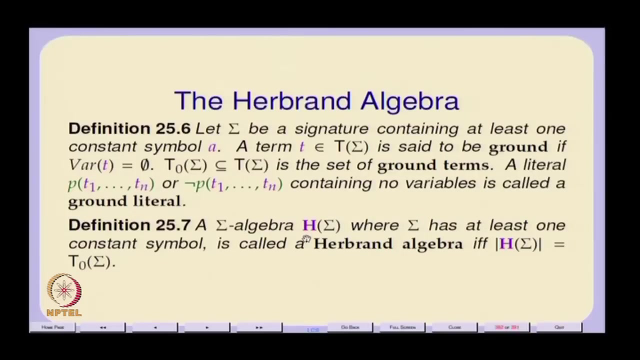 for sigma itself And consider the algebra. instead of considering an algebra sigma comma A, You consider the algebra sigma comma t sigma, And that is a Herbrand algebra here. So we will call that H of sigma. So in particular, the important thing, 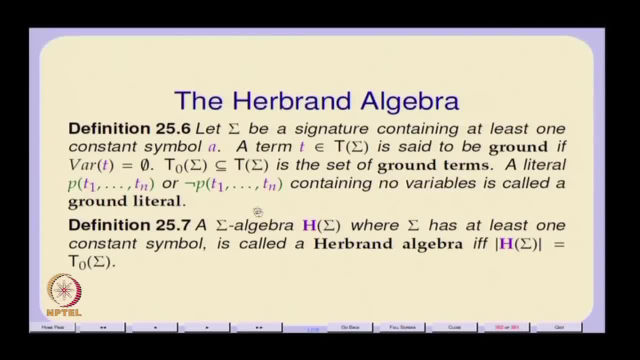 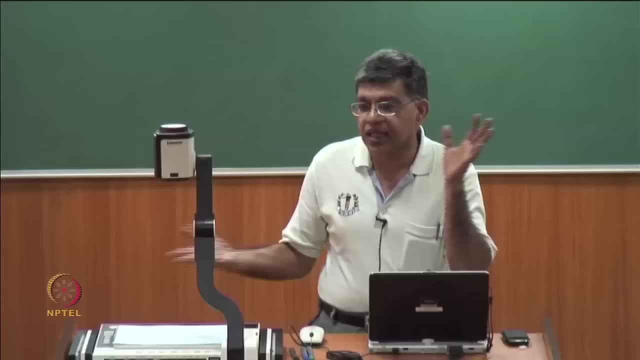 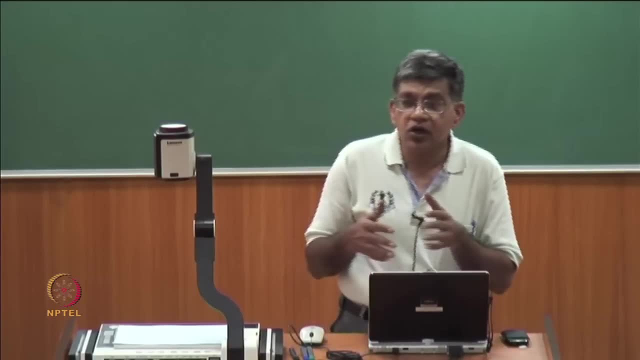 here to realize that there should be at least one constant symbol, because what happens are otherwise is that you are essentially applying functions on functions and functions and functions, and that can be infinite regress. So if you want to have a basis somewhere, there has to be a constant symbol, Since you are not going outside for a model you are looking for. 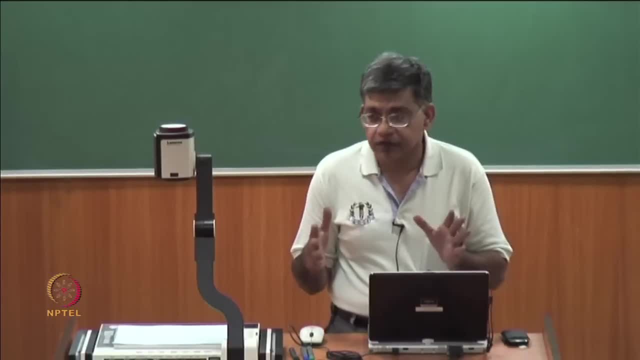 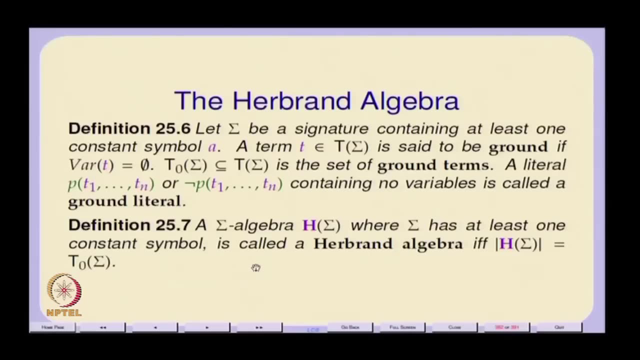 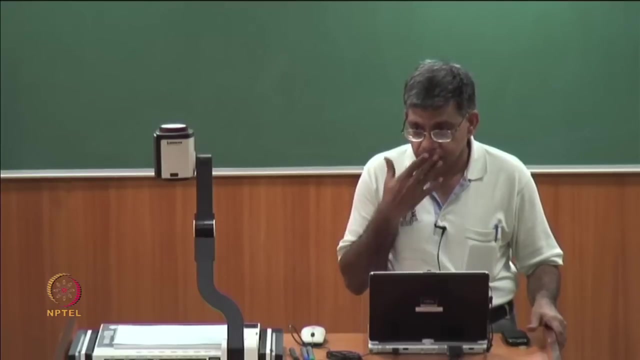 models within the language of terms itself. So we do require some ground terms. if we did not have any constant and there would not be any ground terms, there would only be terms with variables in them, but there would be no ground terms. So that is why this it. 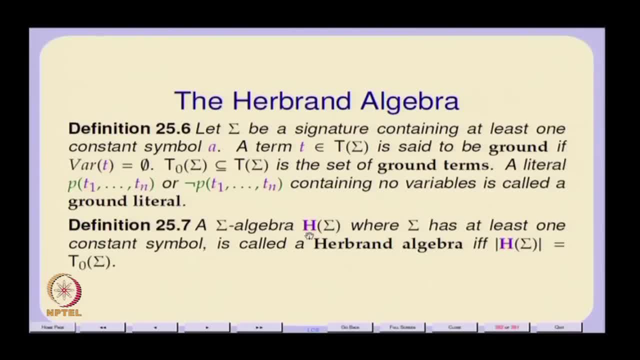 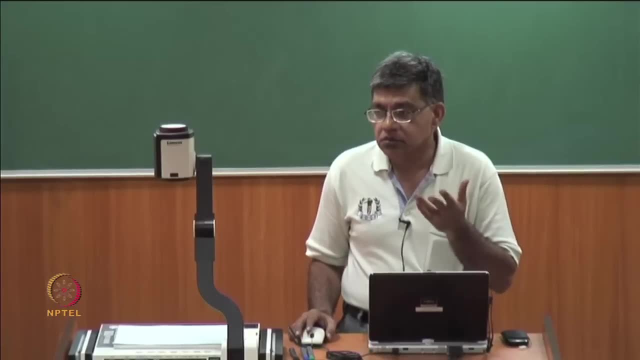 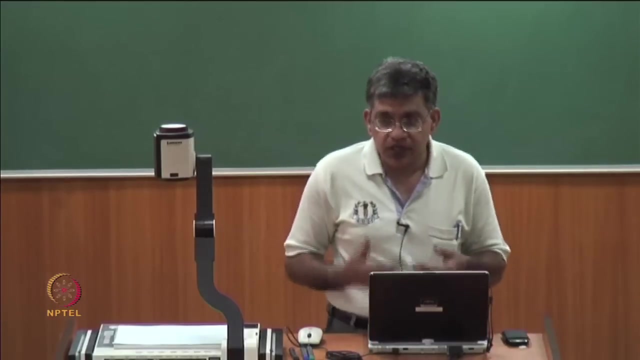 is important to have at least one constant symbol. So it is quite reminiscent of whatever you have done about many of you must have done somethings about freely generated groups, So it is essentially something like that. it is a free algebra generated from sigma. 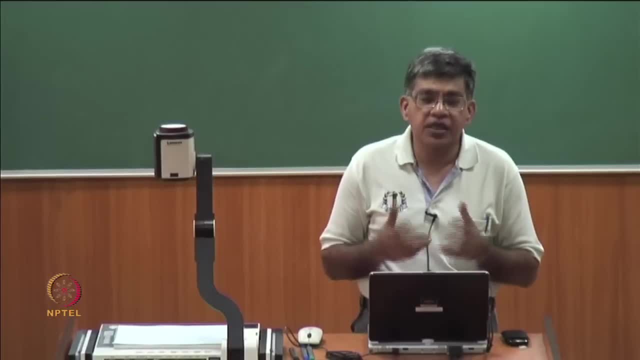 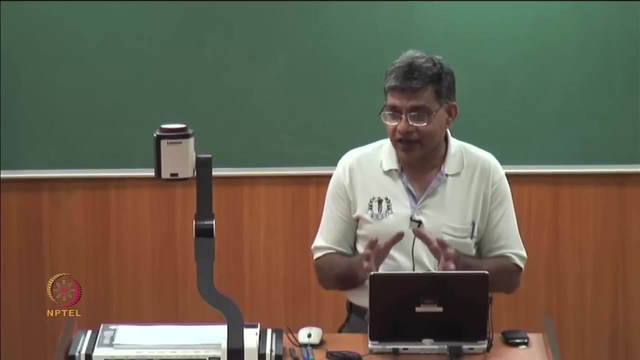 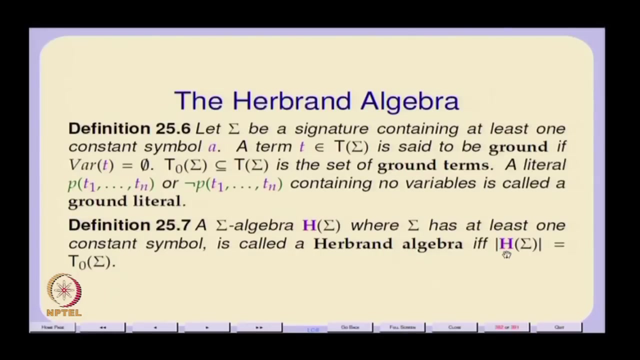 itself. So that basically what I am saying is there is no brown color anywhere. everywhere it is violet. the carrier set is violet in color, it is not in brown. So this is called a Herbrand algebra and it is, and essentially the domain of the algebra are just the set. 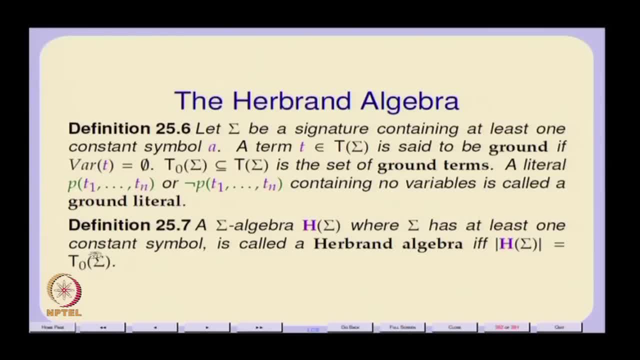 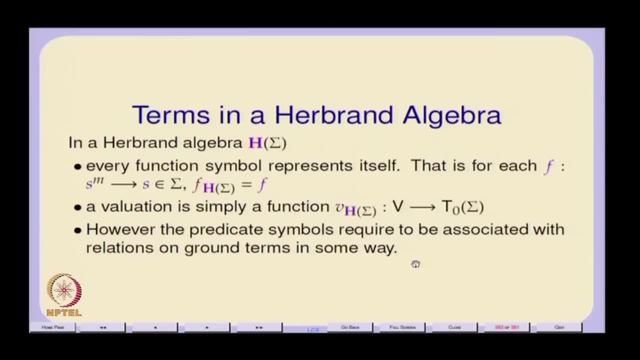 of all ground terms, And if there was no constant symbol, then this set of ground terms would be empty. that is a problem. So you want it to be non empty. So you have this. So you take a Herbrand. 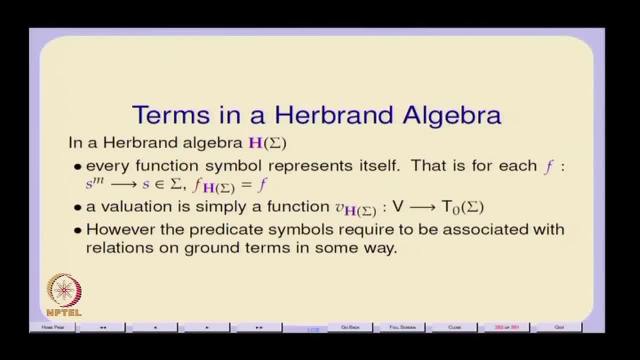 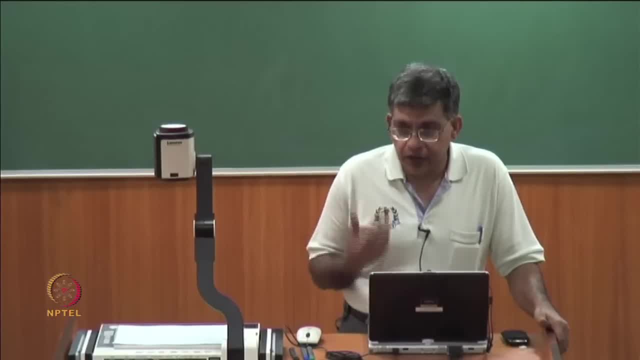 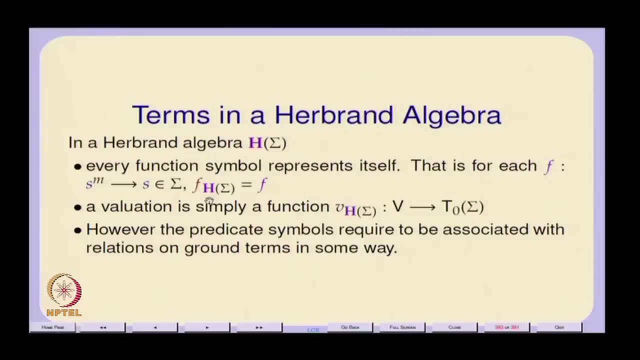 algebra. So now what we can do is now of course we can talk of valuations. So a valuation now will be a function from the variables v to essentially ground terms of this algebra, So for every. So essentially what we are saying is: So I can define, if I can define, 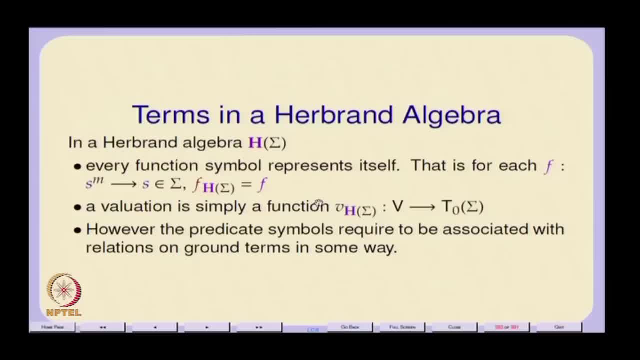 an interpretation over h of sigma, such that every function symbol f in the signature is interpreted as itself in h of sigma And a valuation is simply a function. So you will cups only these three rolls, which associates with each variable a ground term. 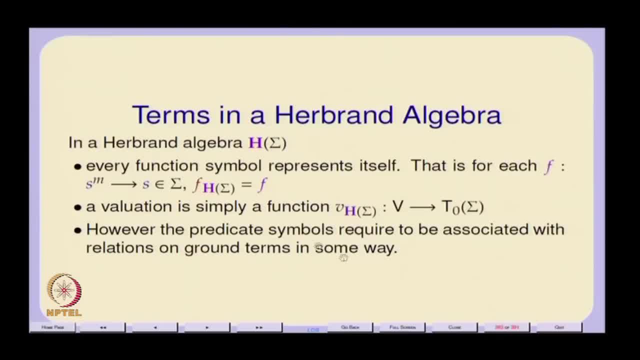 So the only thing, the only difference is that we are not associating anything with the predicated symbols, Right. So at the moment we are leaving the predicate symbols alone. So now a Herbrand interpretation is just: nqu altenavピ k assiminformation kal soll guy. 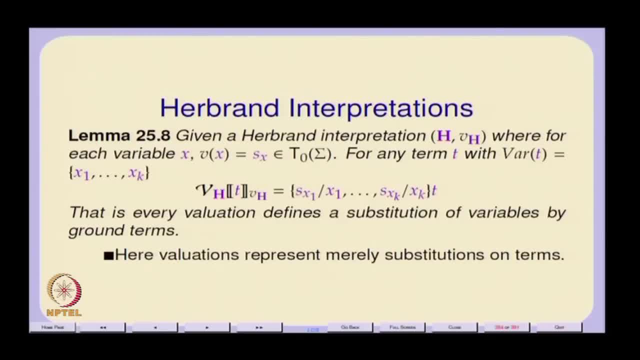 Okay, Okay, algebra. Here I have just a Herbrand algebra. this should be h of sigma, but often I just even the sigma is understood, I will not mention it. And then there is a valuation where for each variable x I have a term, a ground term, that 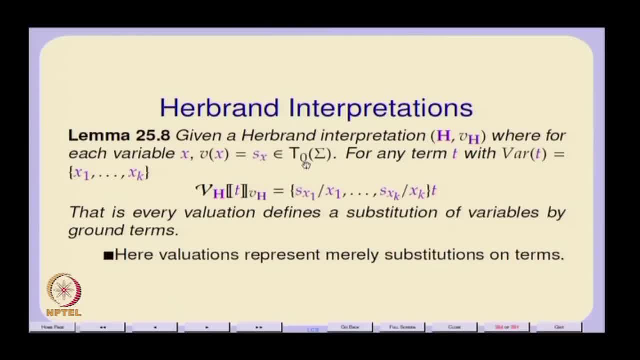 is why it is purple, violet in color, s, x in t, not of sigma. And so for any term t which has variables x 1 to x k, if you were to evaluate this term in this valuation v h, then what you are essentially going to get is a substitution. 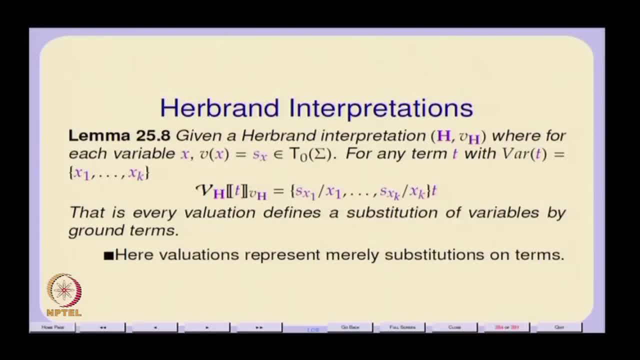 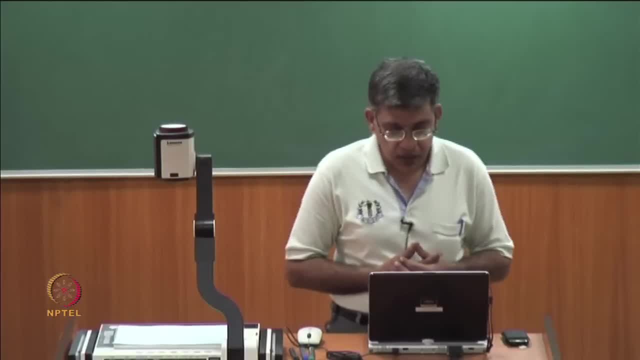 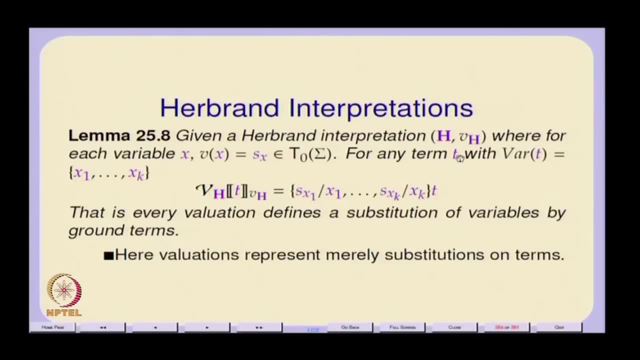 is a pure syntactic substitution, So every occurrence of the variable x 1 will be replaced by the term s x 1.. Of course, s x 1 itself, of course, Because the s x 1 in this case would be a ground term, So it would be variable free. 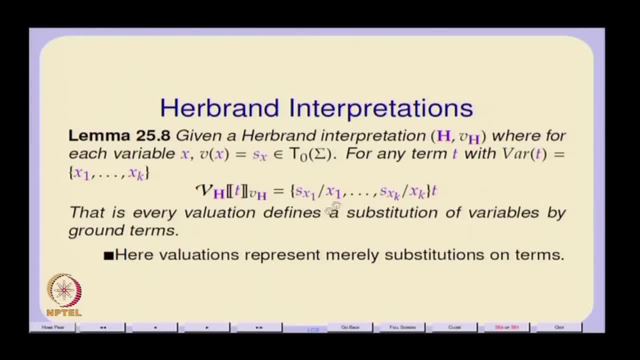 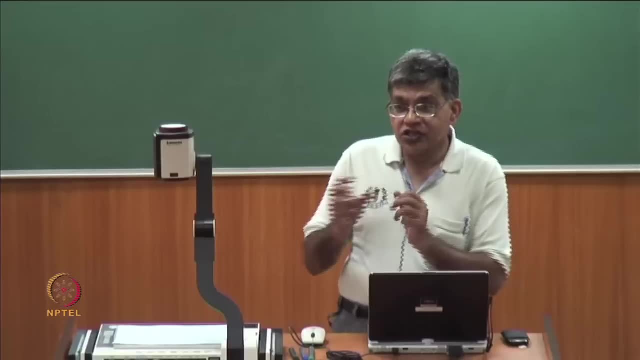 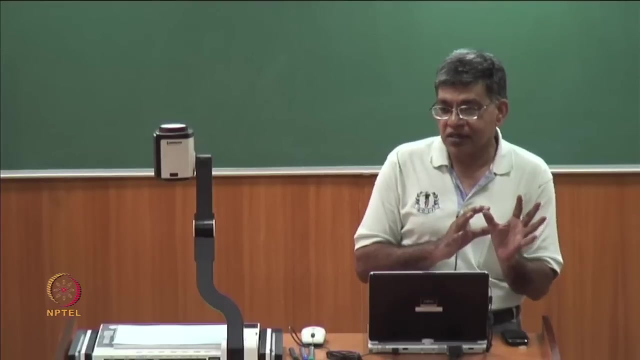 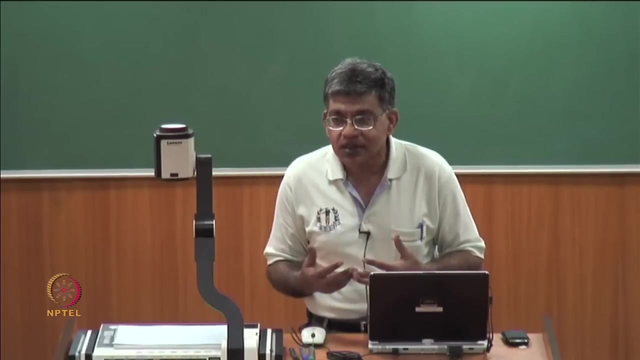 yeah, So what this means is that every valuation essentially defines a substitution. One of the things I did when we did all those coincidence lemmas and so on and so forth, was we showed how variations in valuations are equivalent to substitutions In a certain sense. but now, when your valuations themselves are in the same set of terms, then 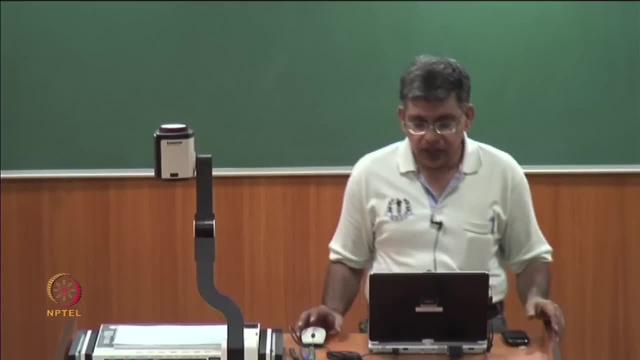 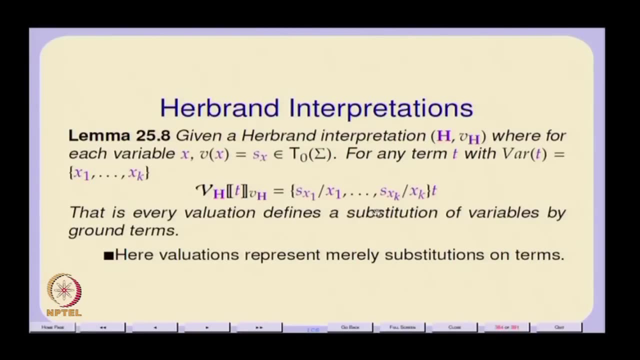 everything collapses to just substitutions. The only thing here is not any arbitrary substitution. it is a substitution of ground terms for variables. yeah, So valuations represent merely substitutions of ground terms, So we would say So. now we have still not actually interpreted the. 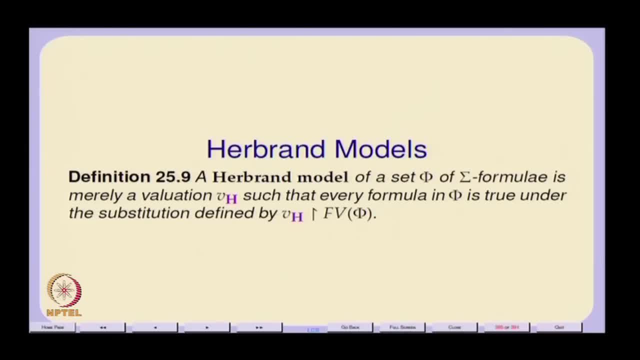 predicate symbols. a Herbrand model of a set phi of sigma formulae is merely a valuation. I mean you can just associate it with the valuation v, h which makes every formula in phi true. And if it makes every formula in phi true then you are not really interested. 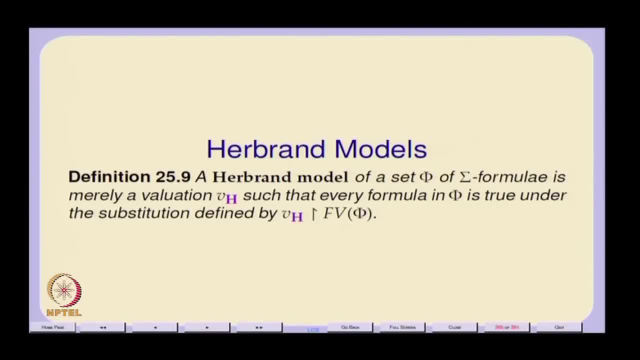 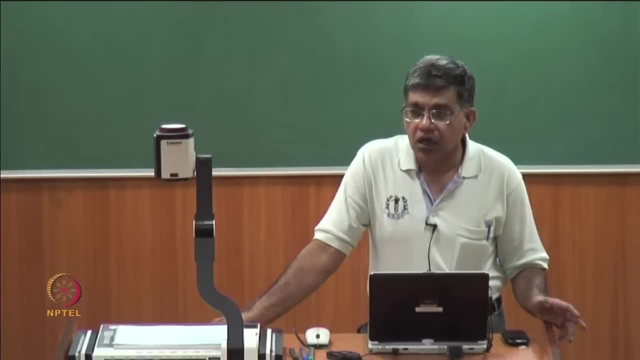 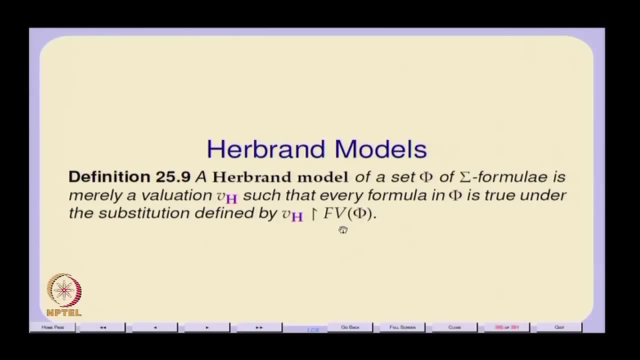 in the finite set of. if phi is in finite set of formulae, then it will anyway only have a finite set of free variables, right? And if it has only a finite set of free variables, then you only need to consider the valuation restricted to that finite set of free variables. So 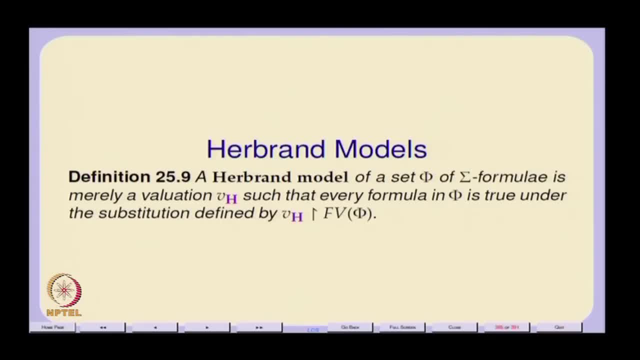 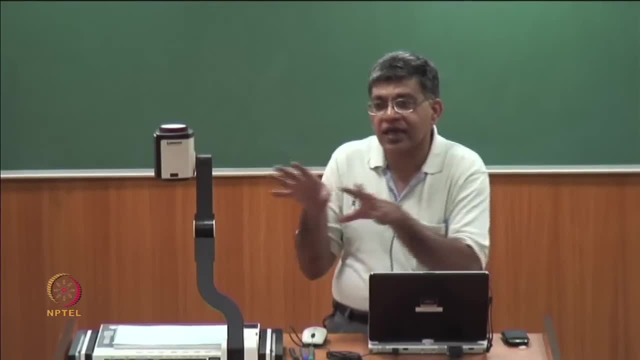 which is essentially a substitution, because a substitution, strictly speaking, is a finite replacement of variables. It is an almost everywhere the identity function. right, that means you have an infinite set of variables, But what you are saying is there are only a finite subset of those variables which are being replaced by. 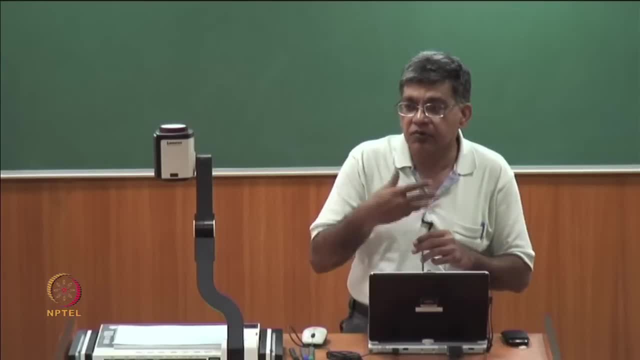 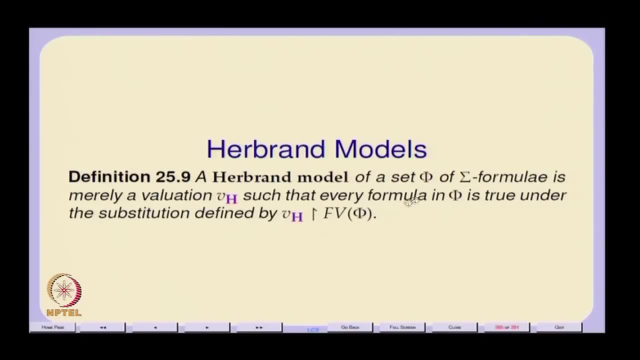 nonidentical terms right Which are not being replaced by themselves. So in the case of any valuation v h- essentially a Herbrand model of a set phi, will be restricted to the substitution created by restricting this valuation to the free variables of phi. 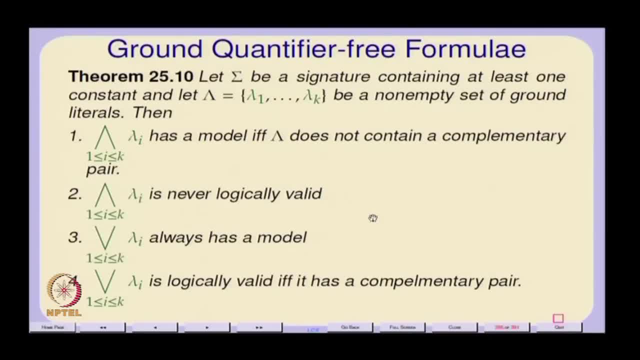 Now, supposing select sigma be a signature, and let us consider a finite set of literals, lambda 1 to lambda k. So these are ground literals, So they are variable, free. So there is essentially atomic predicates on ground terms or negations of 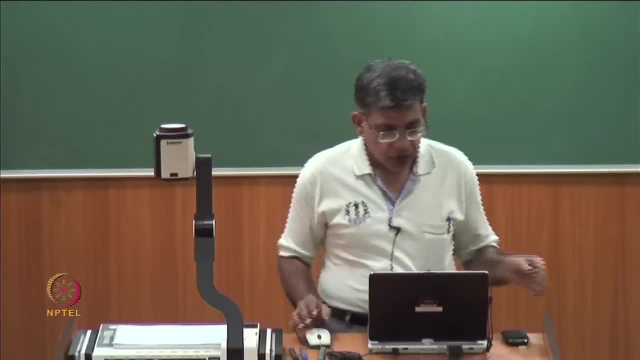 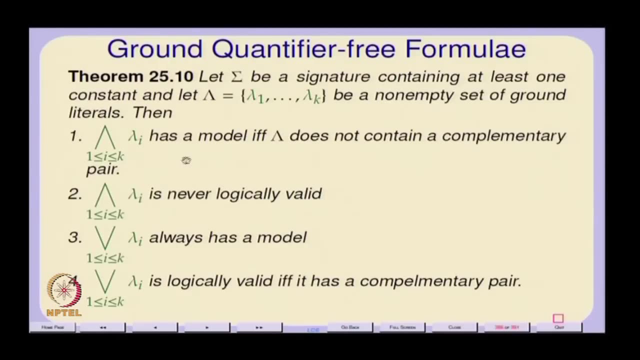 atomic predicates on ground terms. that is what they are. then lambda i has a model, This the big, and of lambda i has a model, has a by a model. we are saying actually we are referring to Herbrand model, But at the moment let us just 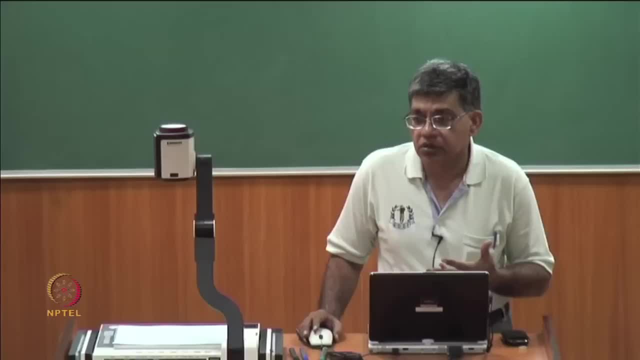 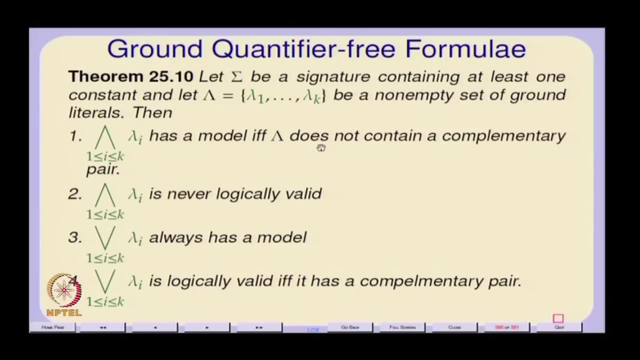 Look at it this way, our proof will actually construct a Herbrand model. So the big and of lambda i has a model if, and only if, capital lambda does not contain a complementary pair. And big and of lambda i is can never be logically valid. And or of big or of lambda i always. 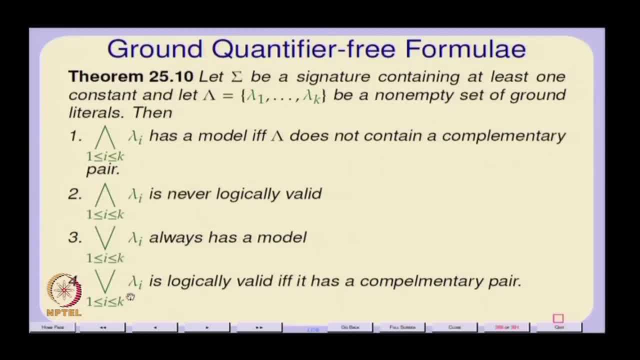 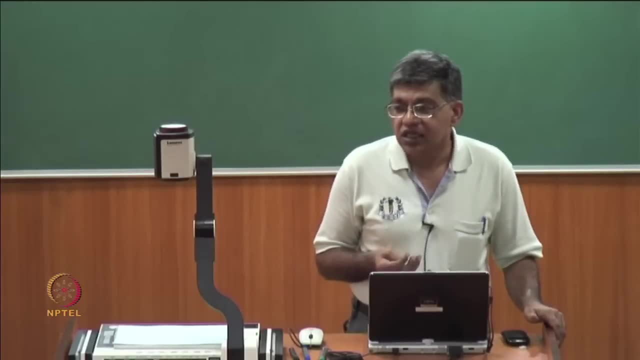 has a model And big or of lambda i is logically valid if, and only if, it has a complementary pair right? The whole point about all this is that in order to look for models for formulae, we do not need to go anywhere else. We could actually look within the term algebra itself. 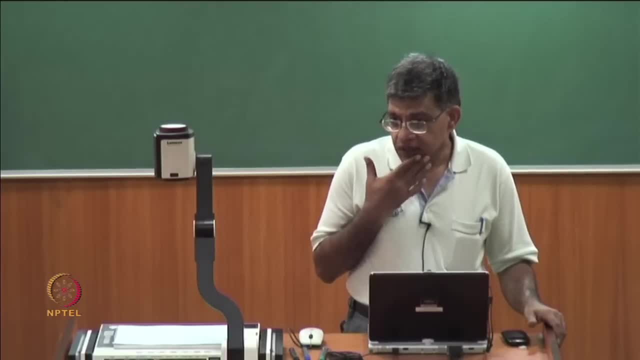 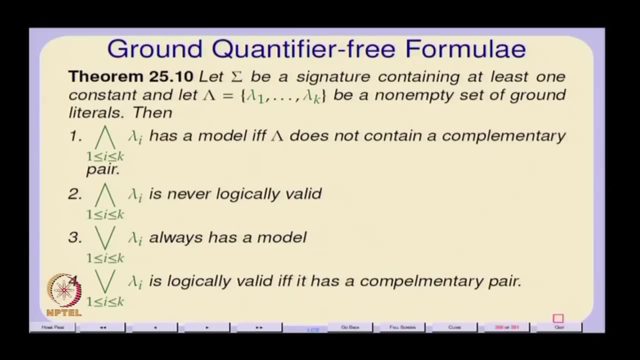 by looking for Herbrand models. So one of the important theorems which I may not do today, But I do not think I can do it today, But which we will use, is So all this, that we 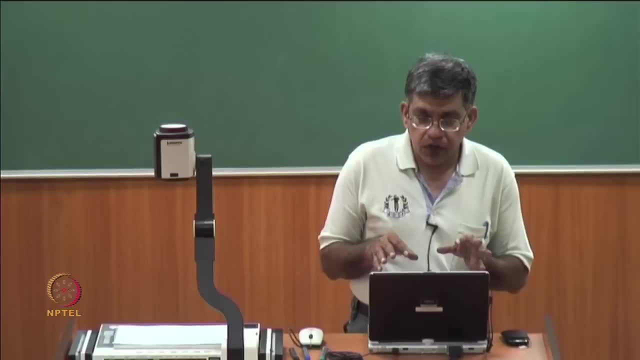 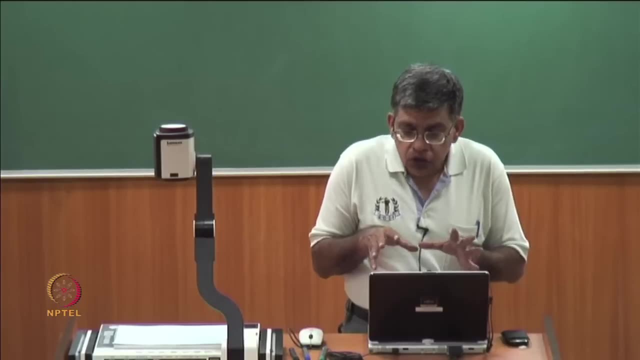 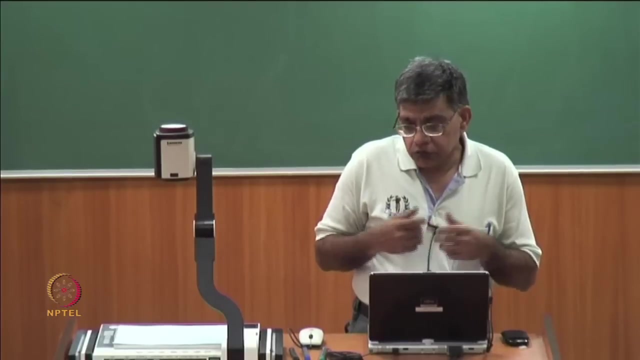 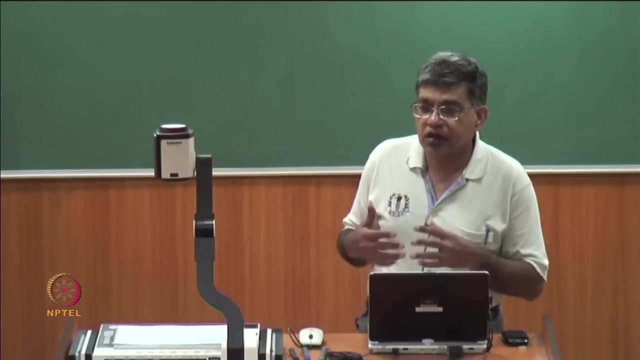 are doing is what leads us eventually to finding, to logic programming. basically, Let us look at it this way: If you have a logic program which has to do some computation, it essentially tries to find some model for the axioms you give it. Now it cannot. no computational mechanism. 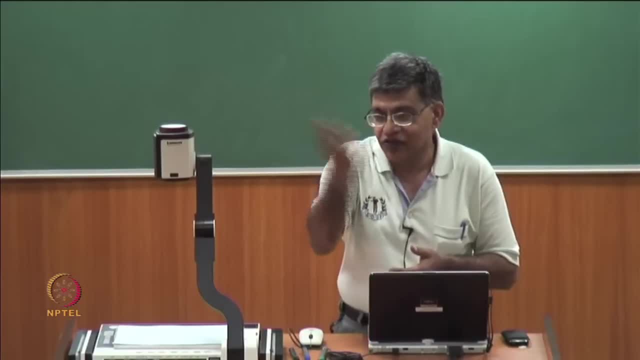 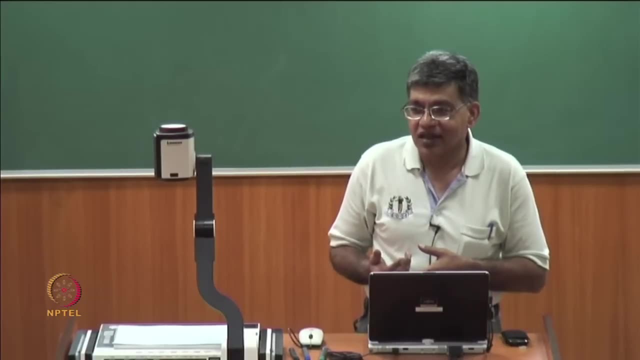 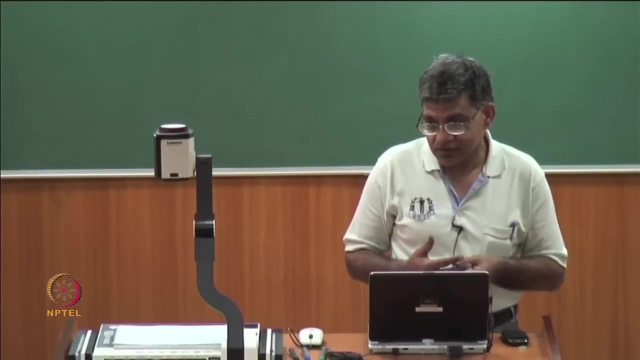 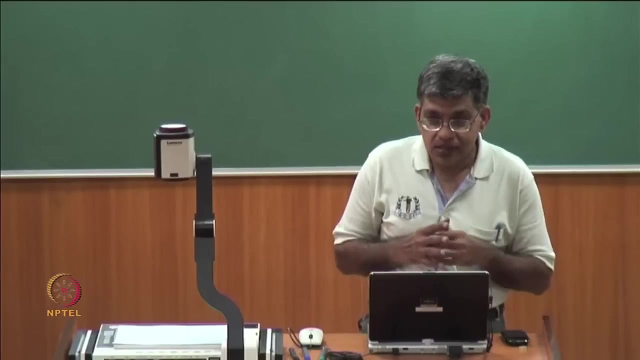 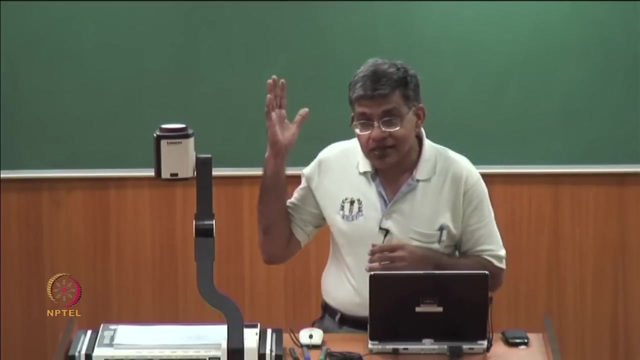 can deal with arbitrary mathematical theories to find models. So it will have to look within itself, within the language of terms itself, in order to determine whether there is a model, And so we require a theorem which says that there is a model in the external world. 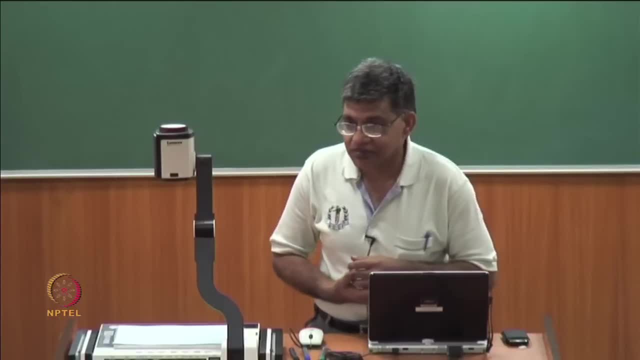 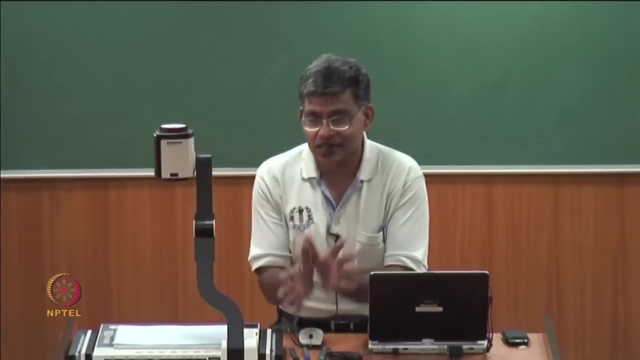 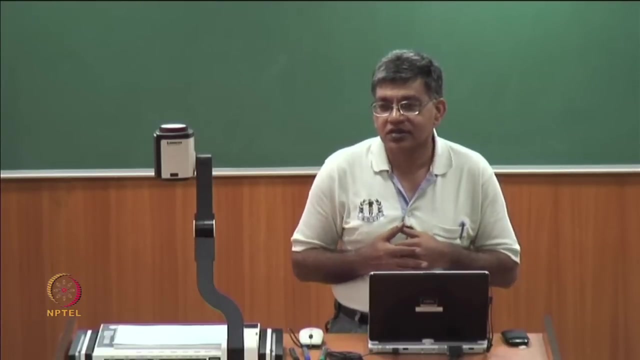 if, and only if, there is a Herbrand model. If you have such a theorem, then what it means is that your computational mechanism needs to look only within itself. It does not have to look outside, in the rest of the world. If your theorem is weaker, which says that if there is a Herbrand model, then there is, 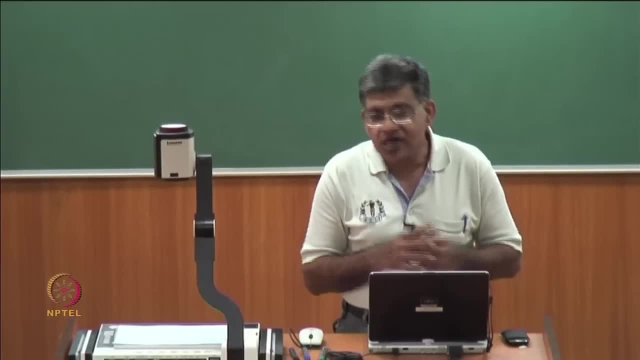 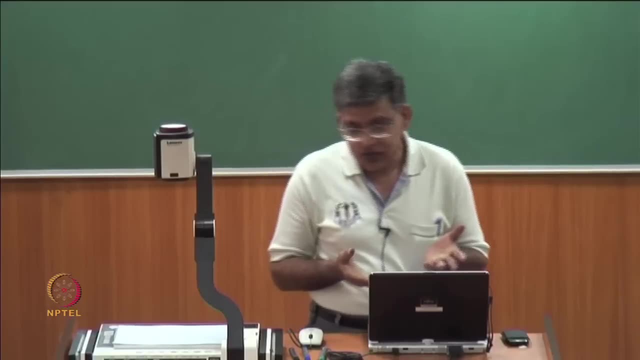 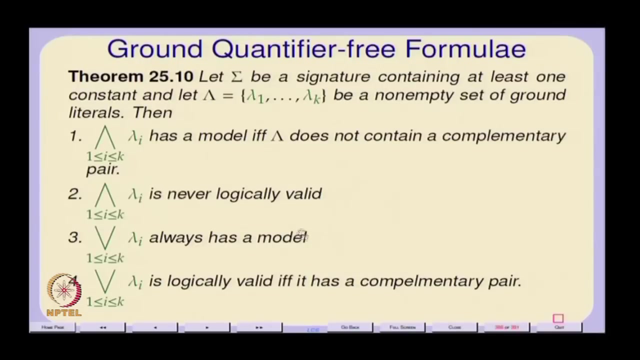 also a model in the outside world, then it is not sufficient, because what it means is that there might be models in the outside world and you may never be able to find a model within this. So this is the first. this theorem is the first step towards. 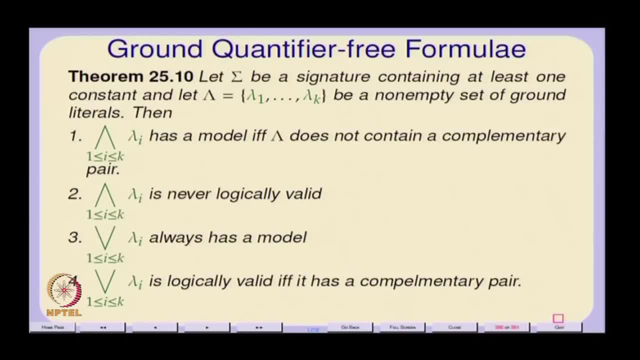 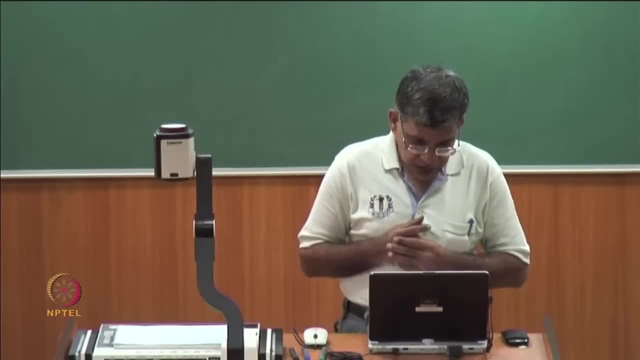 moving towards essentially inward looking models, So what are known as term models. So these Herbrand models in first order logic are in the larger terminology of universal algebra They would be called term models. basically, In a certain sense, all our computations are dealing only. 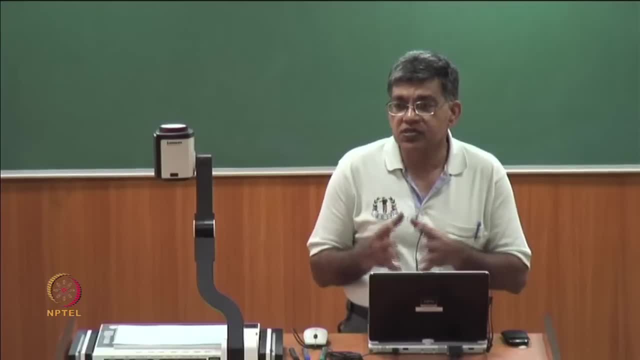 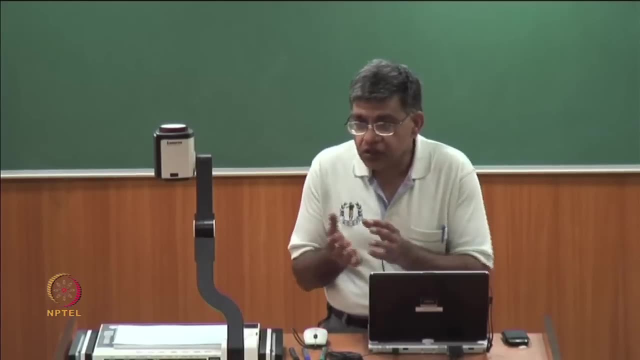 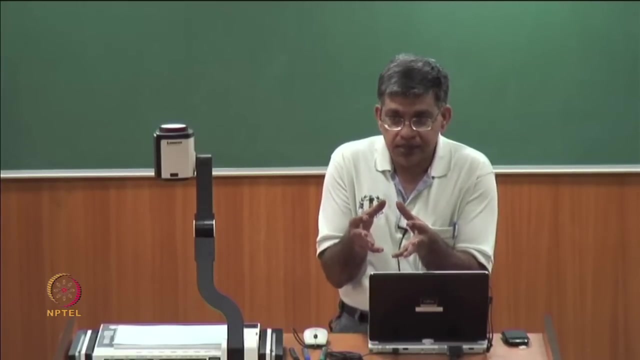 with term models So you can think of them as terms. you can think of all your models of computation involving a machine, Let us say, as essentially looking at that machine as an, as a sigma algebra, where the sigma are all the operations that the machine can. 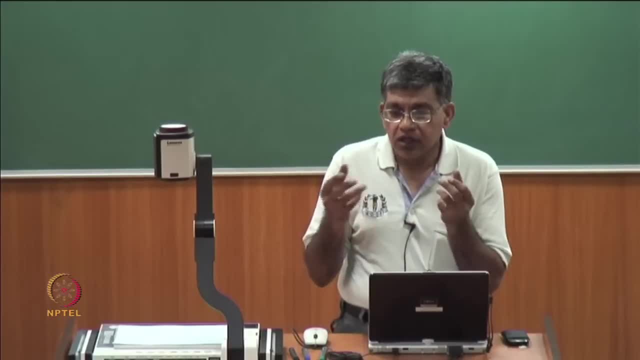 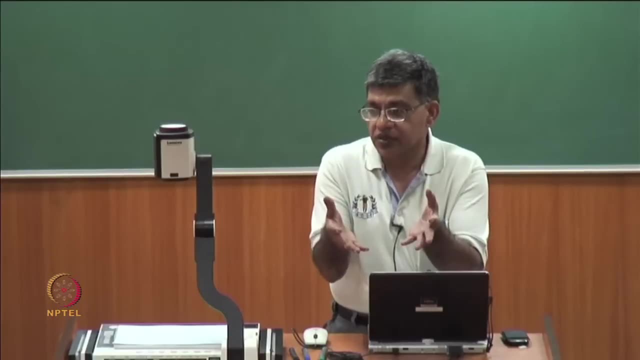 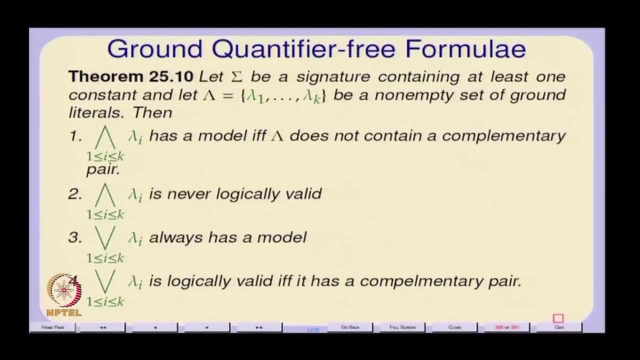 perform And all the expressions that are dealt with are just the terms of that sigma: algebra. So this is a fairly powerful notion, that which actually brings us to computation And in fact it brings us to the notion of computation from logic much later than people. 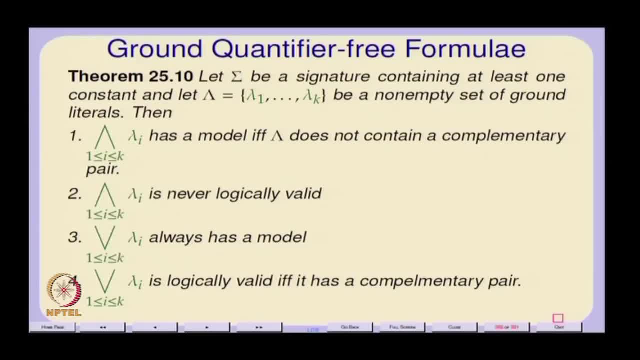 realize. I mean, it is only in the 60s that some- that Robinson- realized that this could be done, though people like Herbrand had actually proved these theorems in 30s. So let us prove this theorem. So what do we have to do in order to? So let us take this big conjunction of 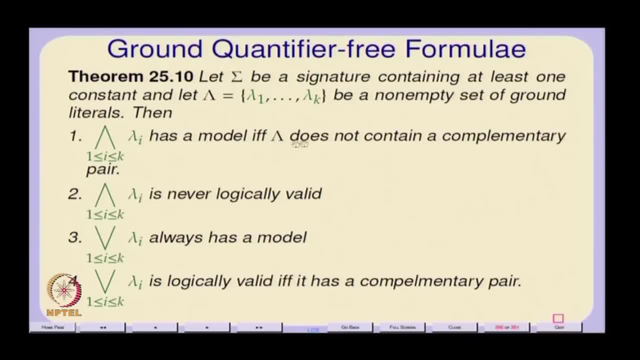 lambda i's. And if it does, if it does have a complementary pair, of course there is no way it can have a model. I mean, it is already, it is already gone, So let us assume it does not have a complementary pair. So if it has a model, then it definitely cannot have a complementary. 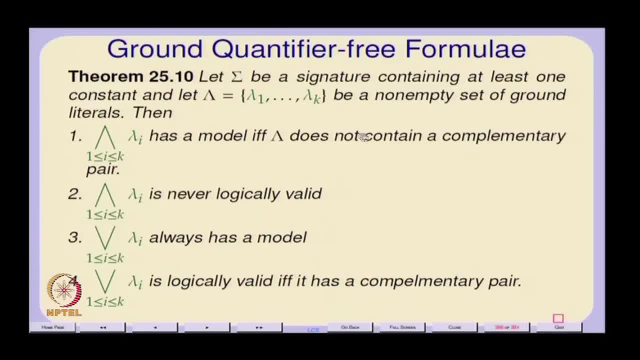 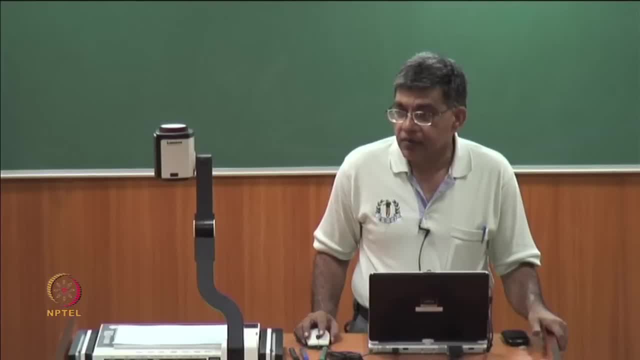 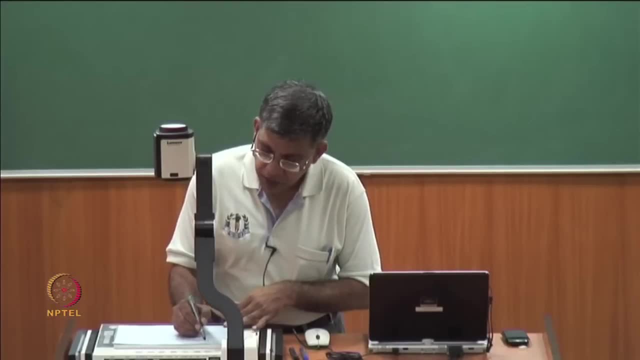 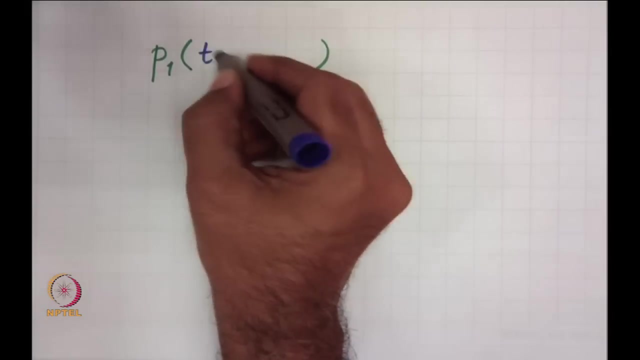 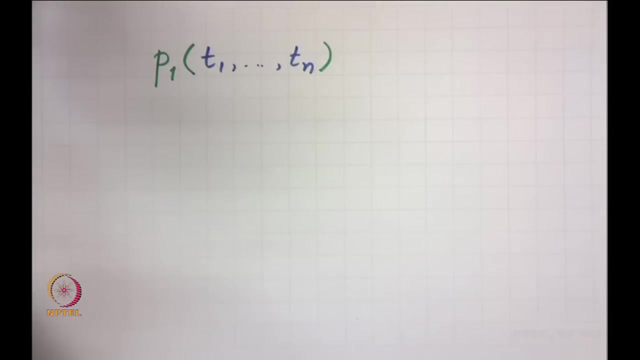 pair. that is one thing. So let us assume that it does not contain a complementary pair. So these lambda 1 to lambda k's, all of them are of the form. let us say some p of lambda 1 of some ground, purple ground terms, right. some p 1, some p 2. something may be of some. 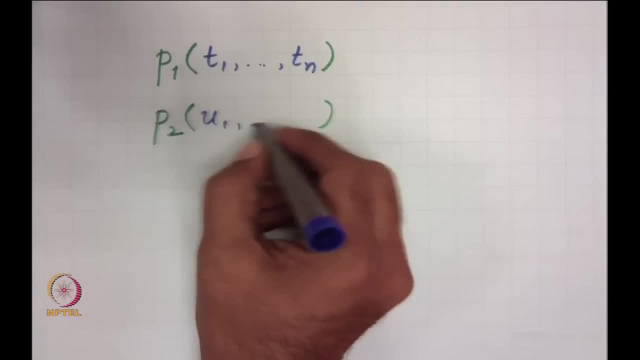 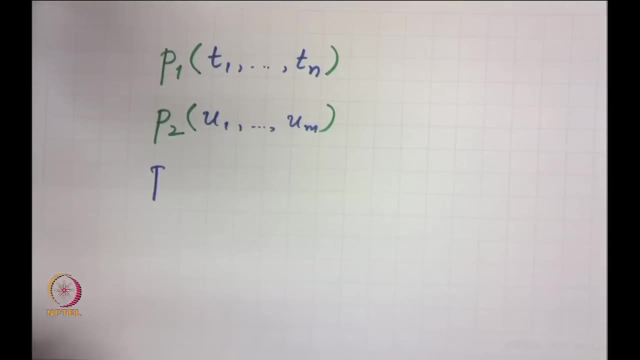 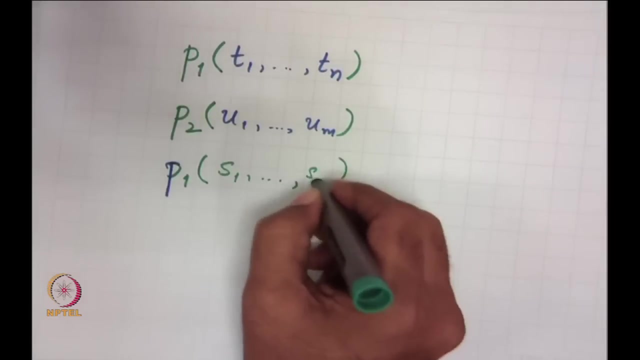 other terms. let us say u 1 to u n. Then may be another one, is, may be just p 1. it is 1 itself, but with some different set of terms: s 1 to s n. So this k could be a very large. 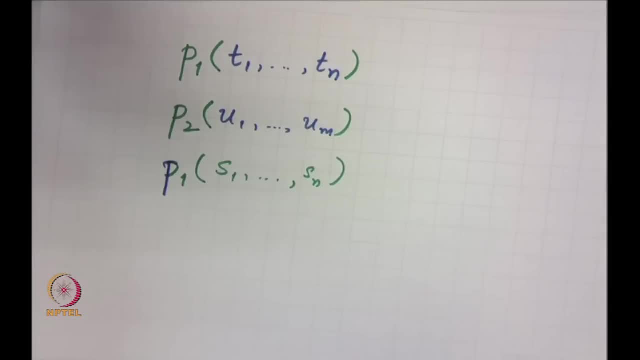 set. I mean this k could be a very large number: lambda 1 to lambda k. So all these lambdas are essentially these. these kinds are atomic formulae, So it should. it could, for example, have this: So you have got a. 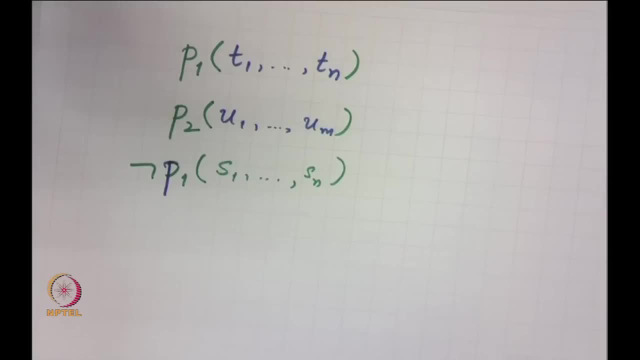 set of. in your sigma you got a set of atomic predicate symbols with their arities and you have, you take various, and you take your lambda 1 to lambda k is constructed out of various ground terms. I mean, this is somewhere ground literals, So they are all ground terms which 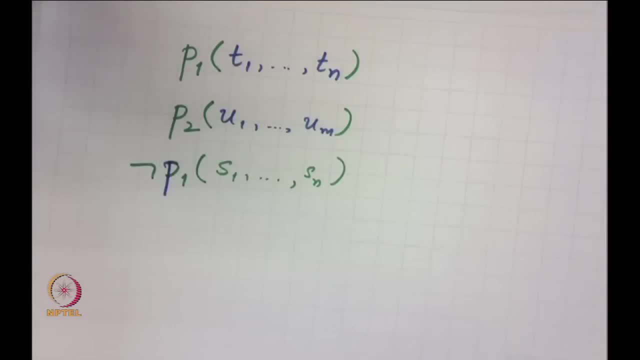 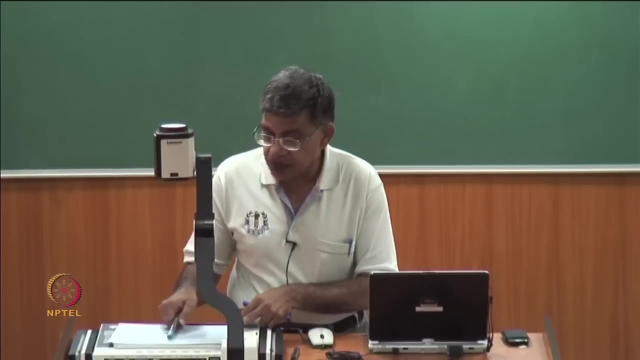 means they are completely variable, free. Now, what you are saying is- and you are saying that there are, there is no complementary pair. Note that if s 1 to s n are different from t 1 to t n, clearly this is not a complementary pair. We have moved away from. 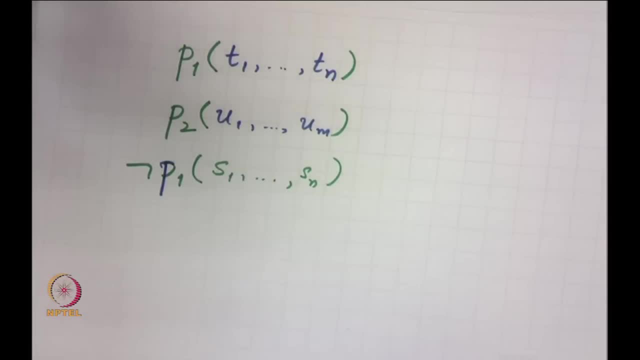 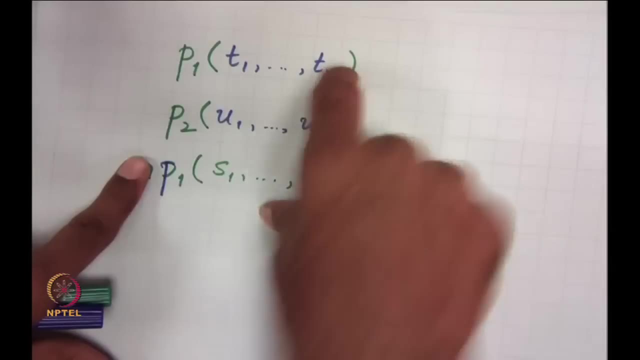 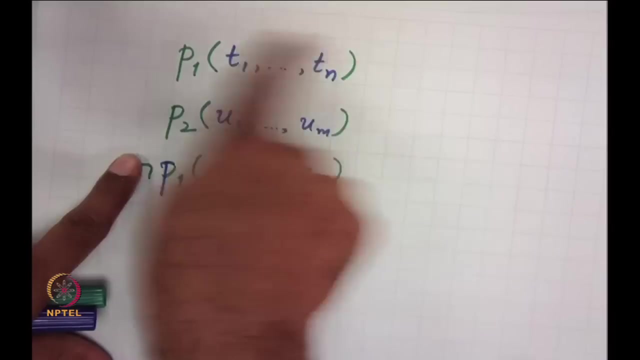 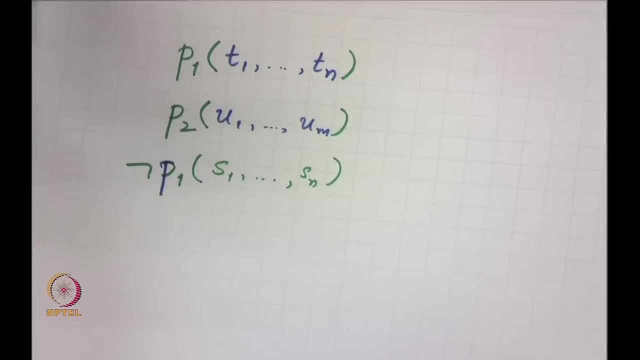 propositions, to parameterize propositions. So a complementary pair. these two would be complementary pairs if only if they looked exactly identical, if they had identical abstract syntax trees, or rather this was an identical abstract sub tree of this formula right, Otherwise they would not be complementary pairs. So complementary pairs: the parameters. 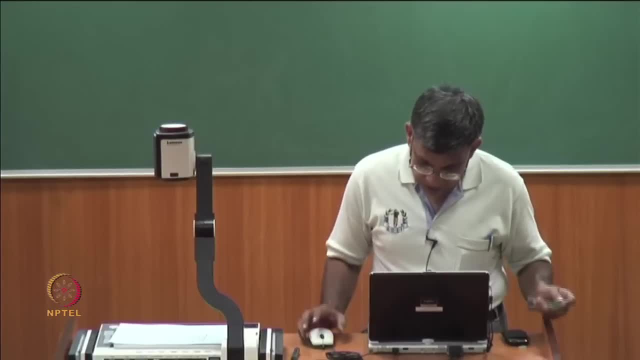 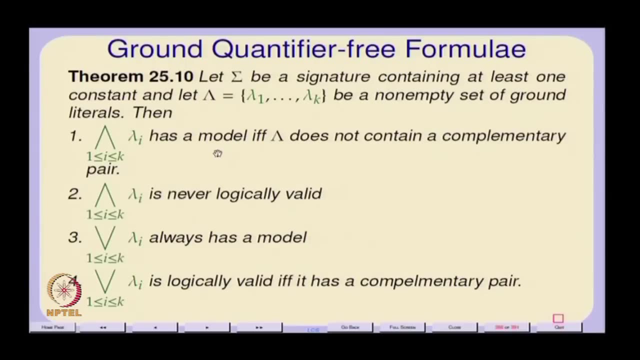 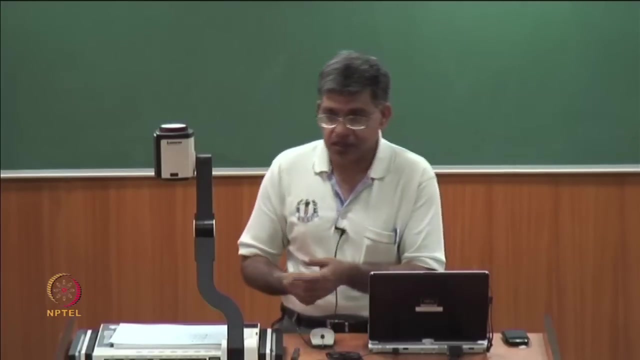 should also match. So then, what do we do we? essentially, we have to create a model, and we are going to create the model as a Herbrand model. So we are going to create a model of within terms itself. So our model is going to be entirely purple in violet in color. 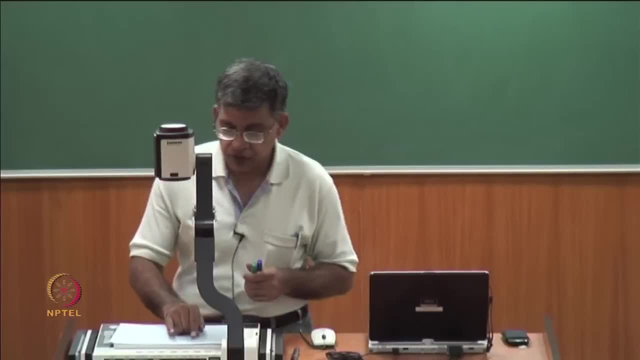 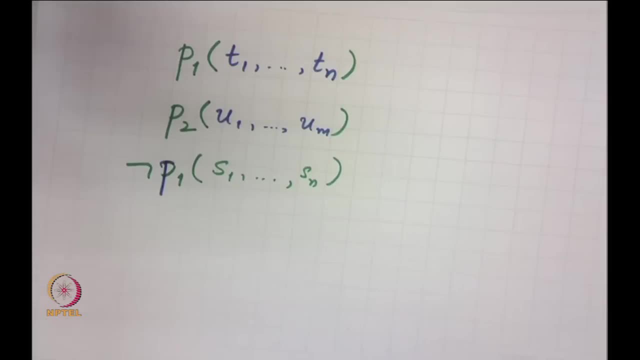 So what we do is we take such, we take this tuple. supposing this is one of the lambda i's, Then our model actually should give me: define a relation right p 1, h, let us say, should actually be a subset of. 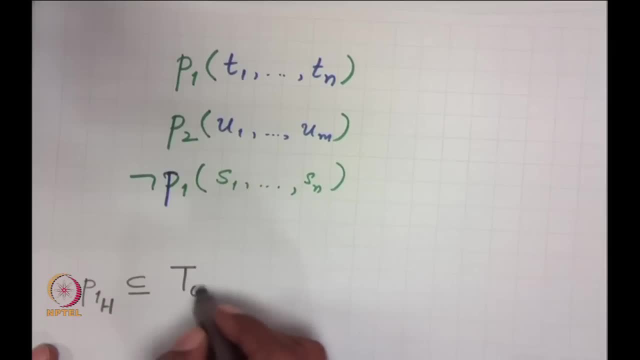 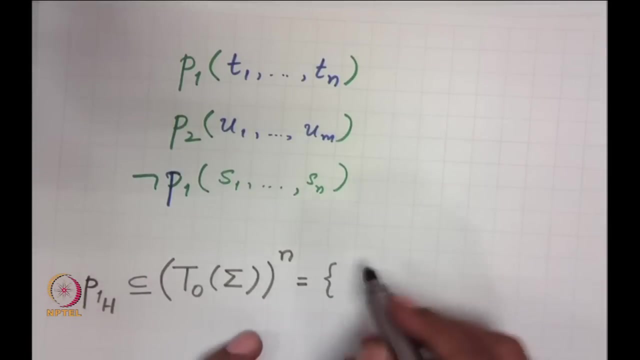 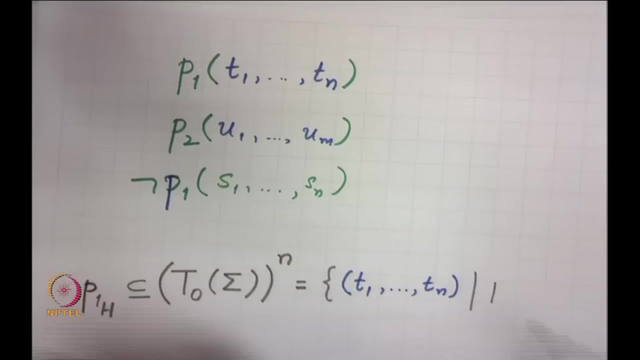 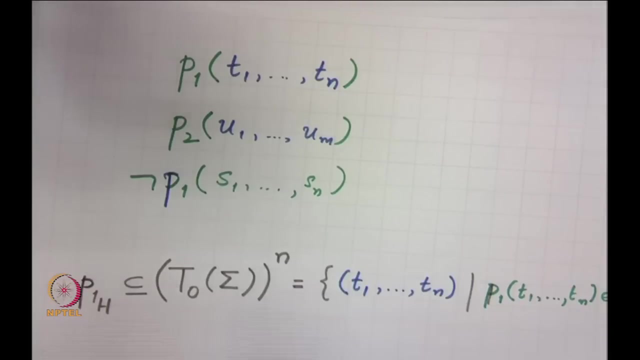 you take all these n tuples of terms where So? for example, you could also have some other. 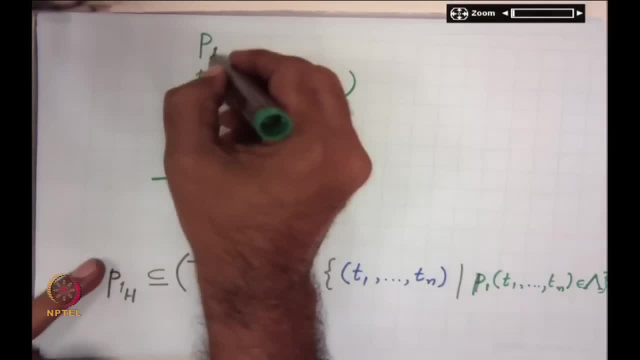 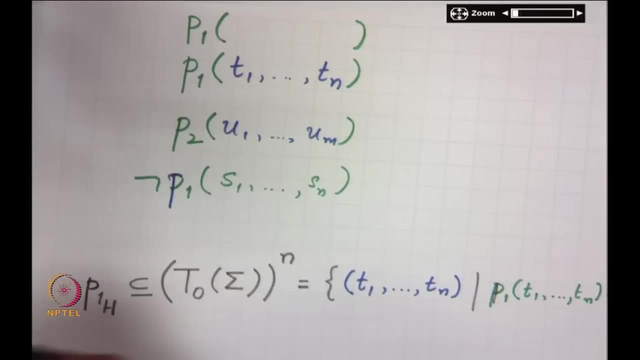 term. you could also have another term with the same atomic predicate also occurring in positive form, which is some term of, let us say, r 1 to r n, where r 1 to r n are terms. So essentially what we are saying is: from this set the, our interpretation of p 1 will. 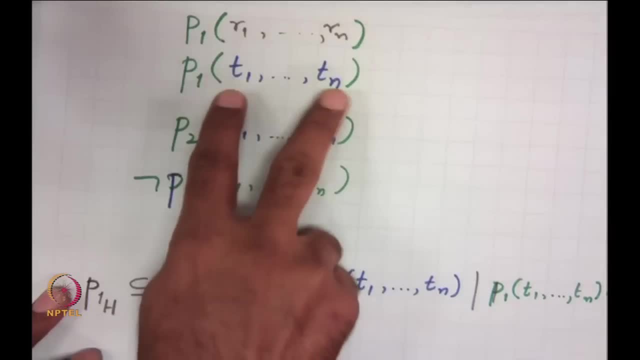 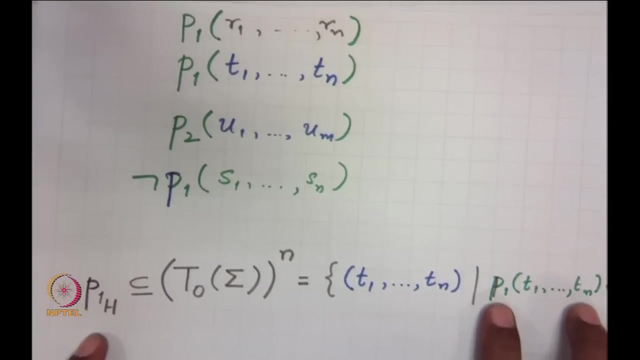 contain these two tuples, r 1 to r n and t 1 to t n, But it is not going to contain the tuple s 1 to s n. that is important to realize that. So for any formula, that so essentially any literal that occurs positively in lambda, 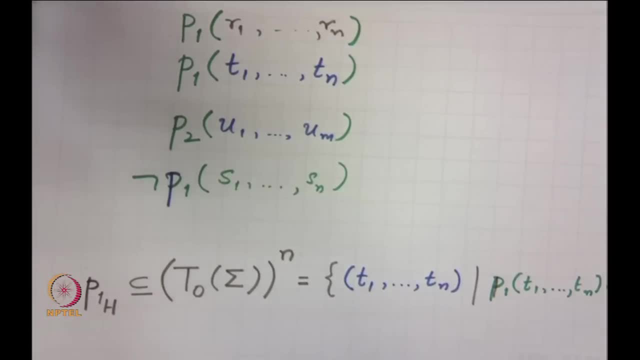 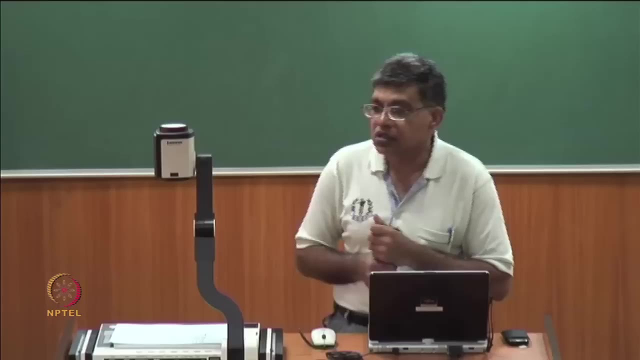 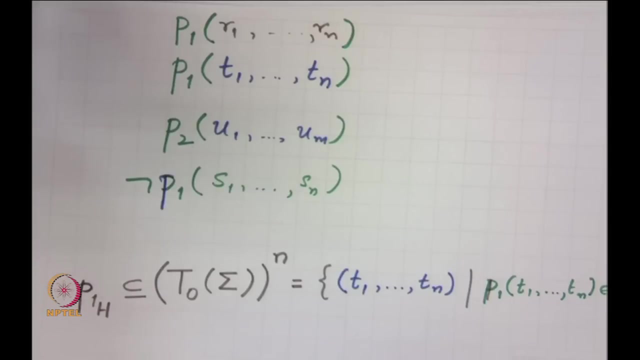 It is parameters which are ground, literals which are ground terms. they are included in the interpretation of that, in the meaning of that relation, of that, the relation corresponding to that atomic predicate. So this is how we construct. So now, this is a Herbrand model. 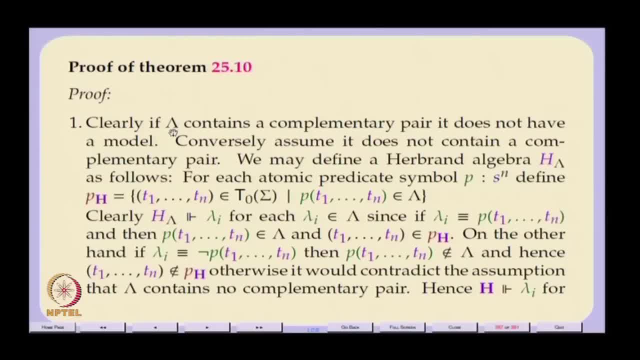 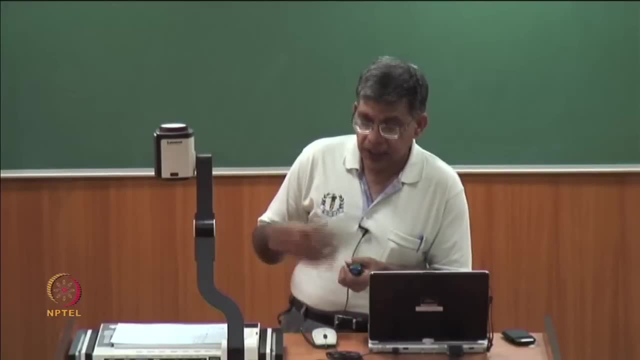 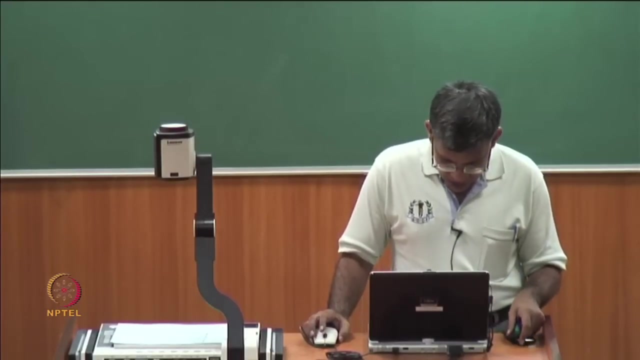 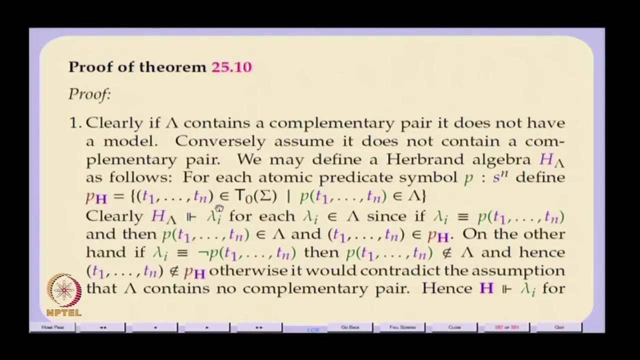 of this set: lambda. this is how you take. you take any literal in this set, you can show that this is Lam, and so you can see this entire interpretation at this algebra is a model of that literal. So that is essentially, am calling this: h lambda satisfies lambda i or a consumption. 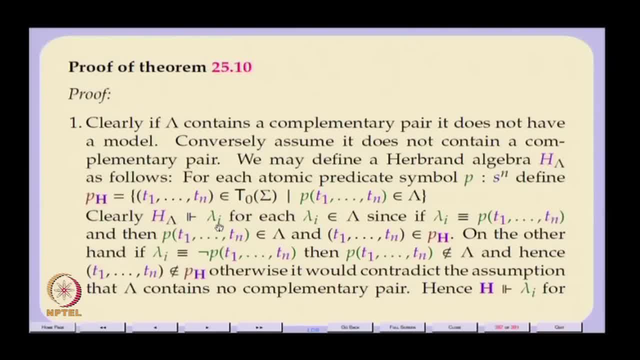 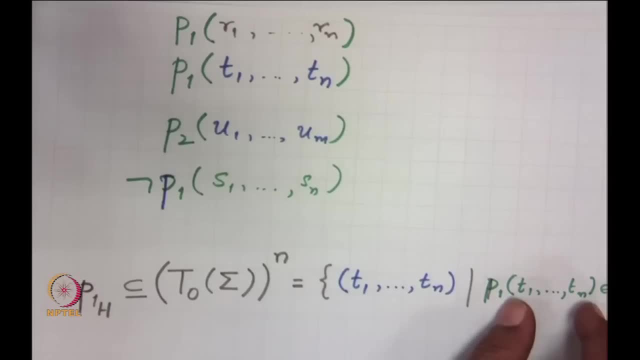 h. lambda is a model of lambda i for each lambda i. So there are only two possibilities for lambda i. lambda i occurs in positive form like this, then it is. parameters are there in the model and So it is true if lambda i occurs. 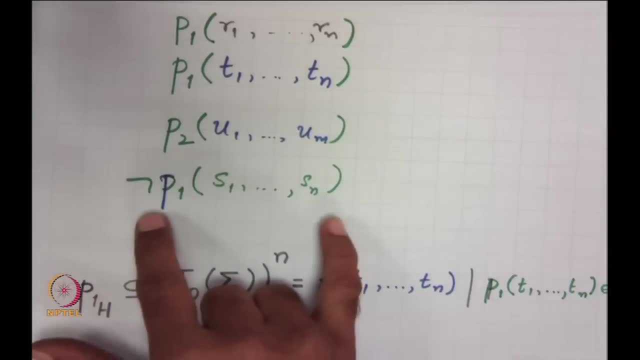 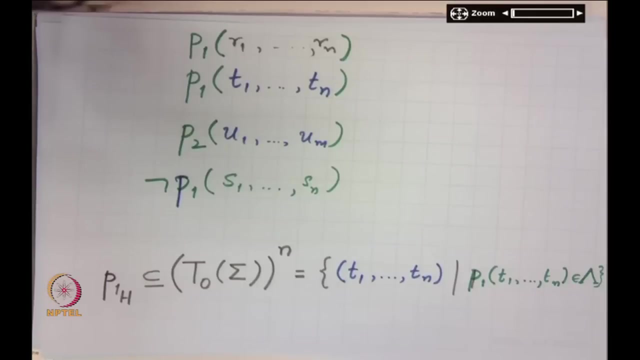 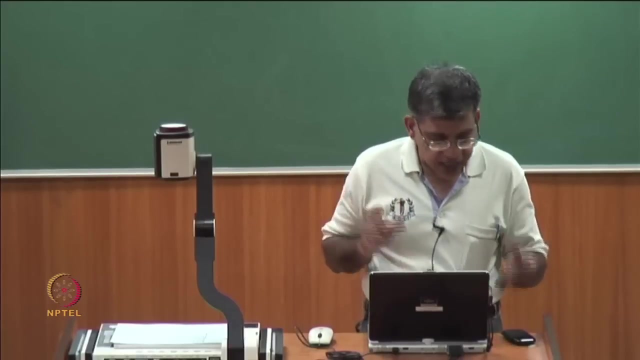 in a negative form like this, then of course it is. parameters are not in this. So therefore by the semantics of the predicate not p 1 of that tuple is true. So every literal lambda i is modeled by this h lambda. what is there? 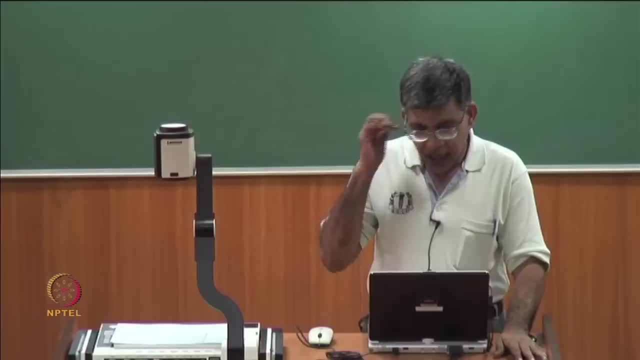 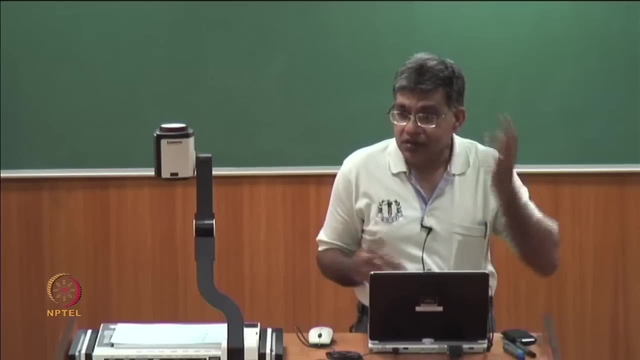 in h lambda. the only thing new in h lambda is that h is already a Herbrand model. So anyway, the terms are t naught sigma. there is no valuation now, because we are anyway talking about ground literals. So it does not matter what valuation you have, the only. 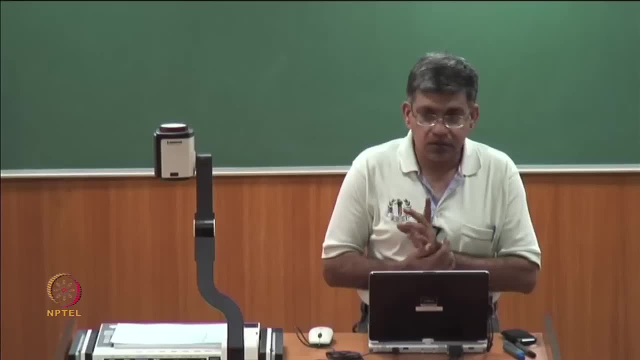 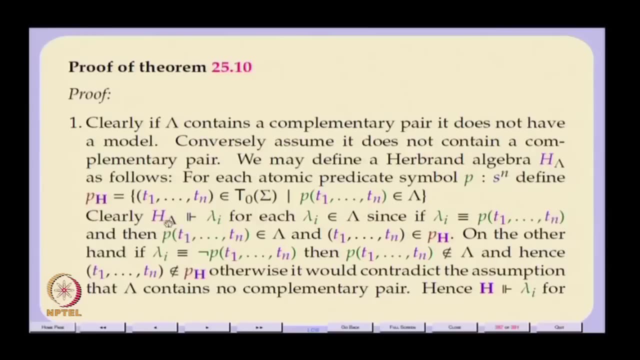 thing you need to do is to interpret the predicate symbols, and So we interpret the predicate symbols. So every lambda i is modeled by this h lambda defined essentially like this. So the relation p- h for each atomic predicate symbol p contains the tuple t 1 to t n. only if p t 1 to t n is a formula, is a ground literal in. 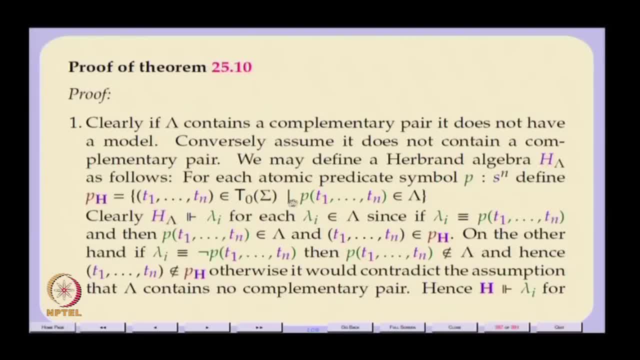 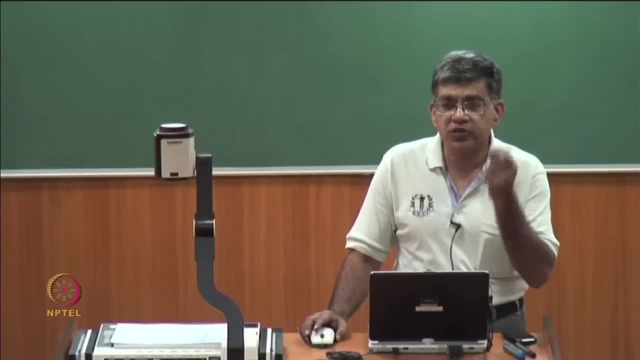 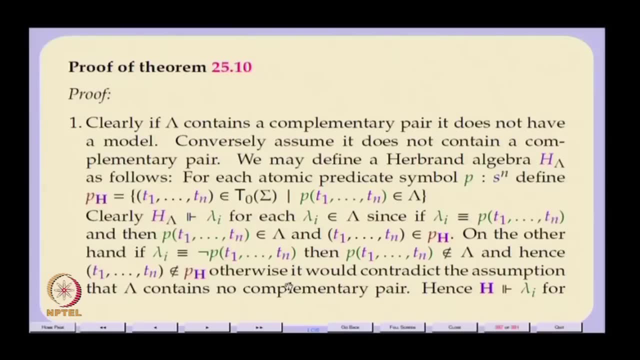 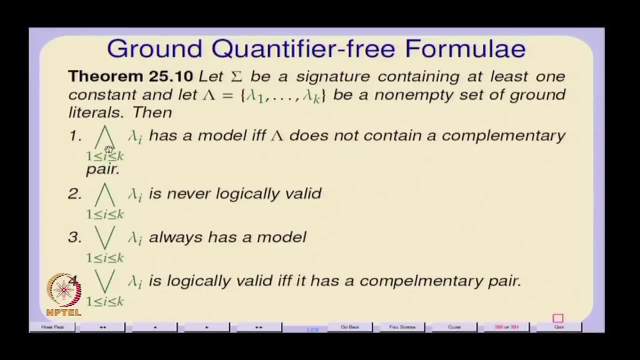 lambda. that is it So? essentially, you ignore all the negative literals, consider only the positive literals and interpret them as the tuples, as their parameters, as being in the relation. that is it So? if so, this h lambda models every lambda i. therefore, it also models the big wedge. 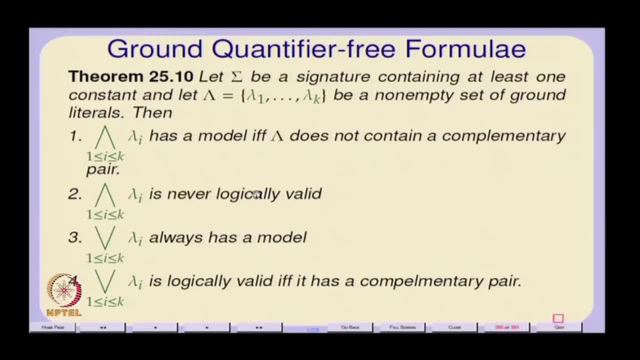 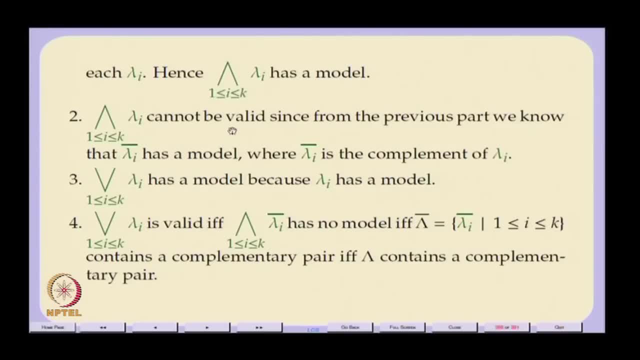 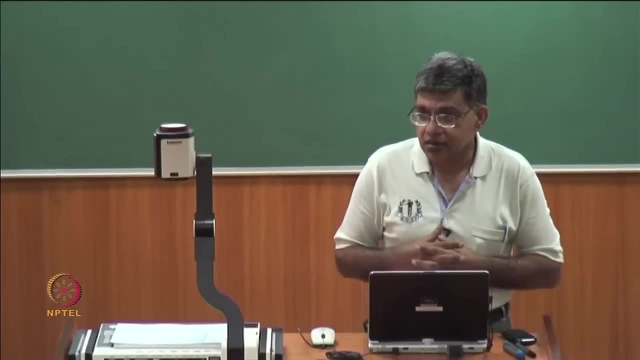 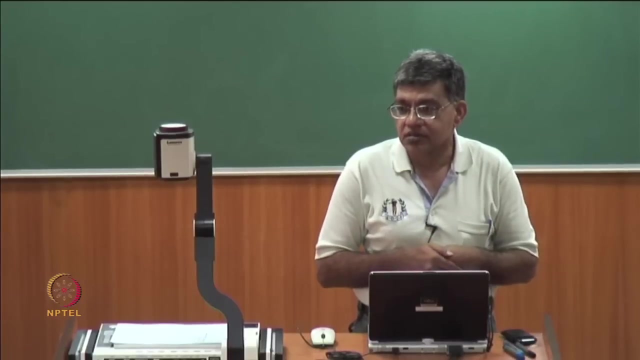 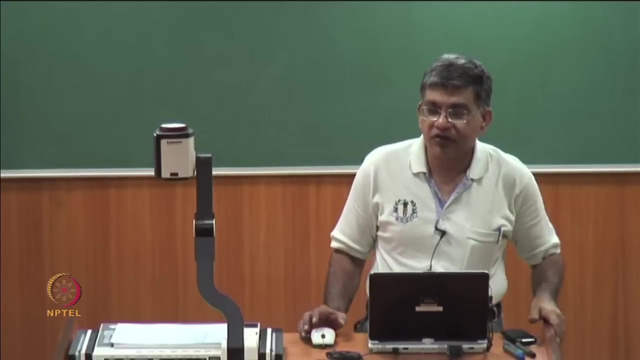 the big and of this lambda i's. 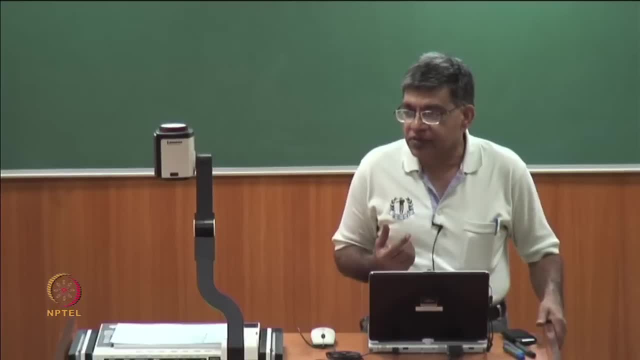 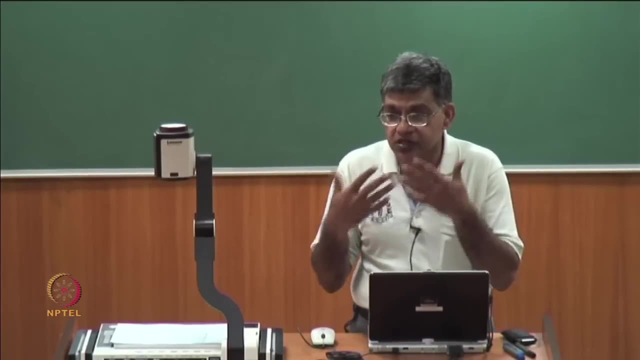 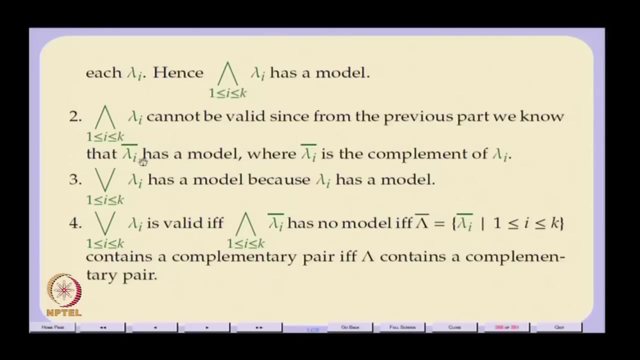 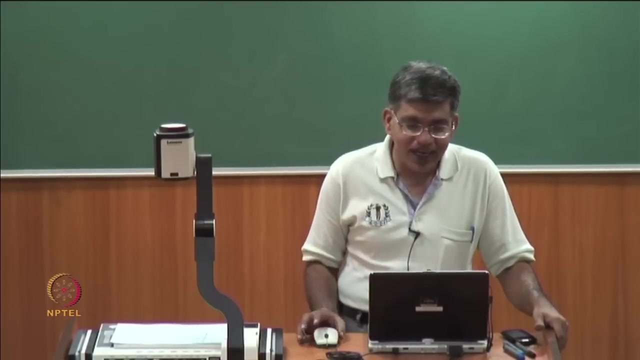 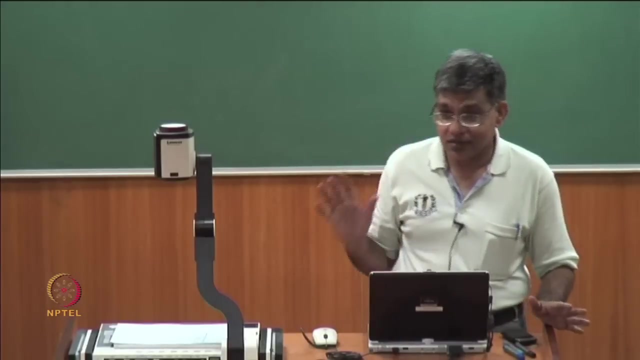 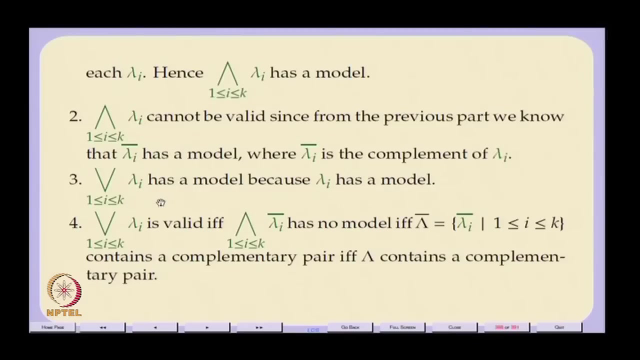 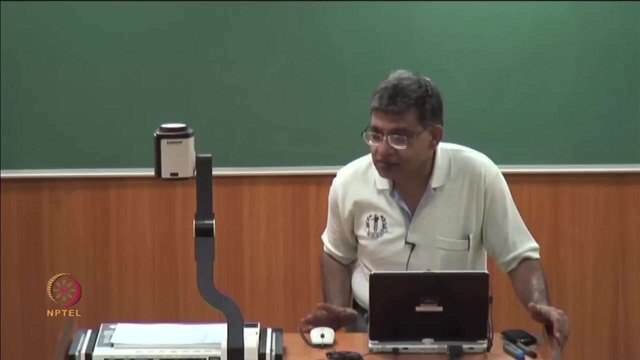 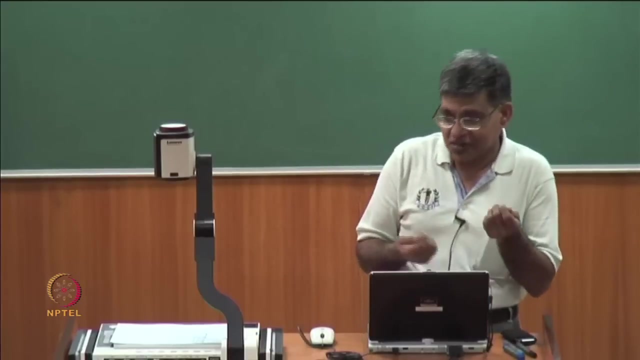 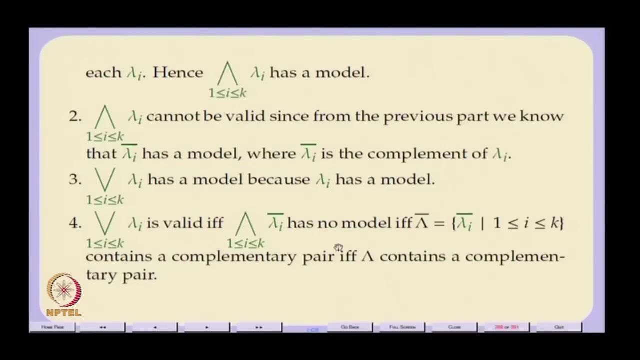 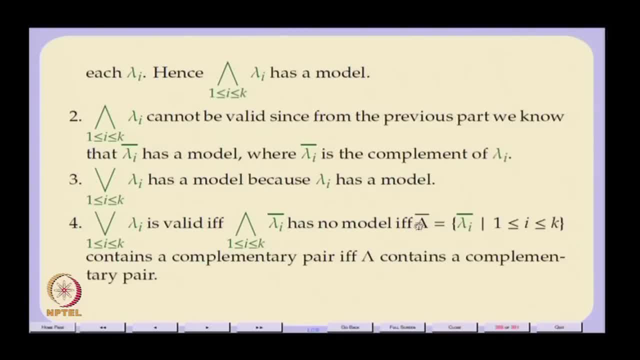 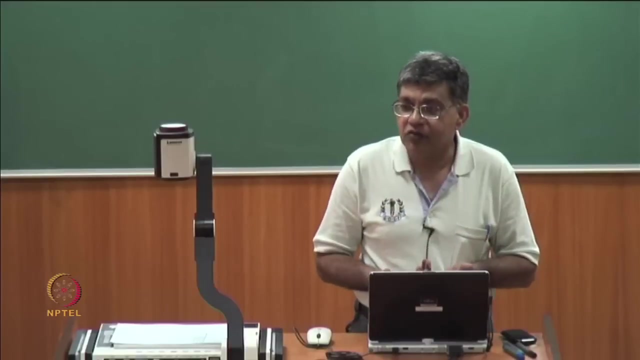 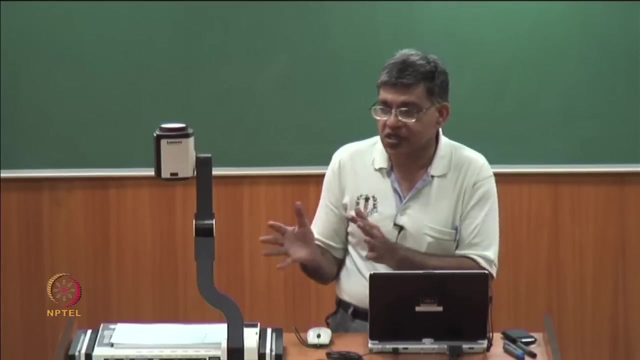 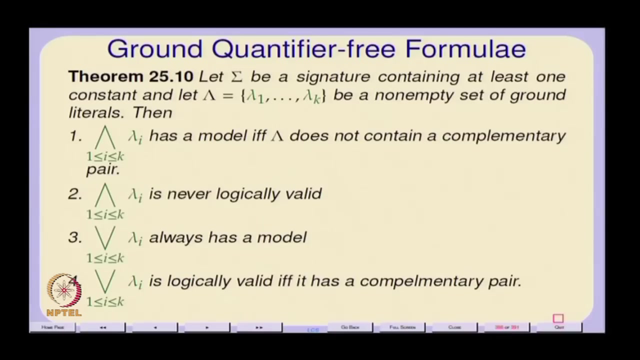 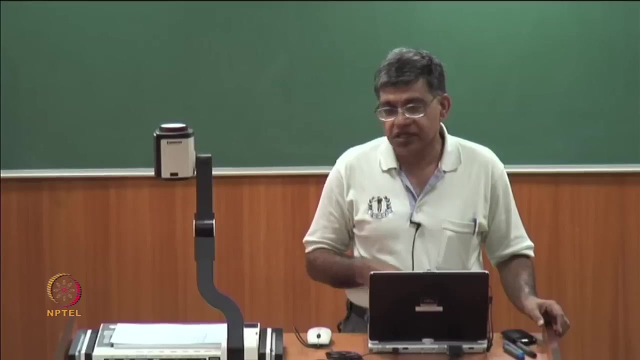 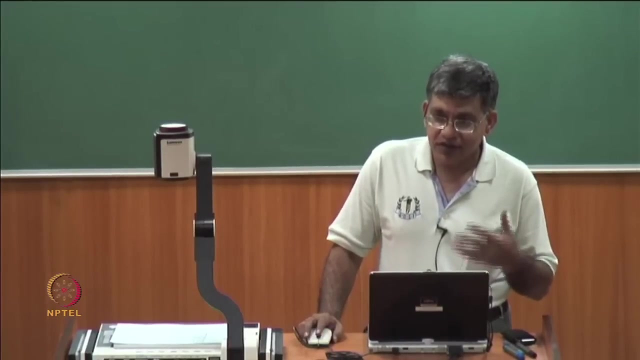 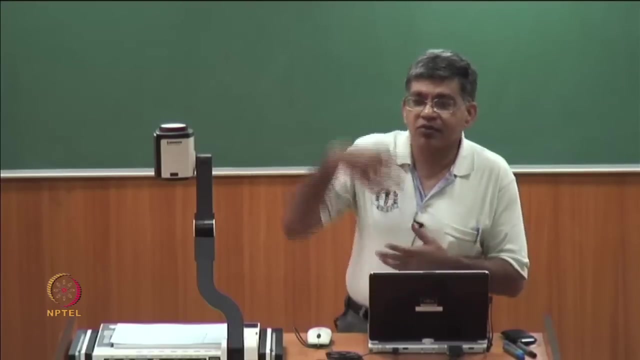 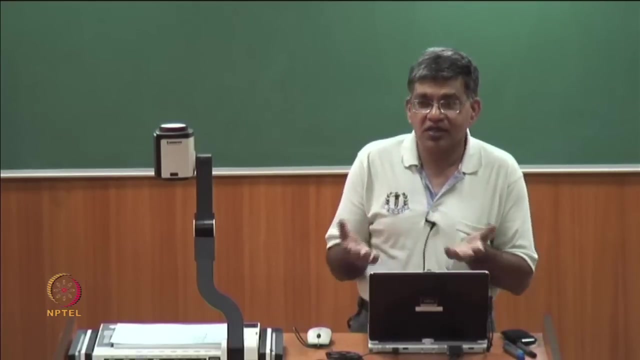 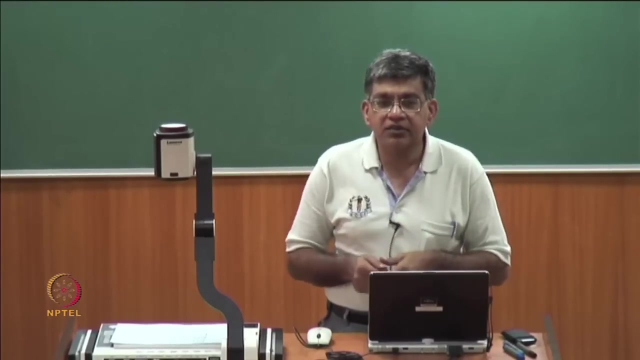 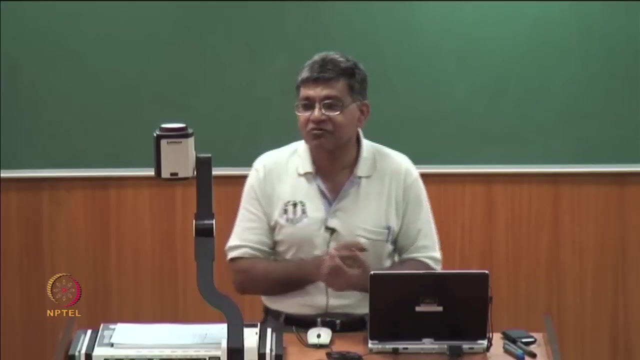 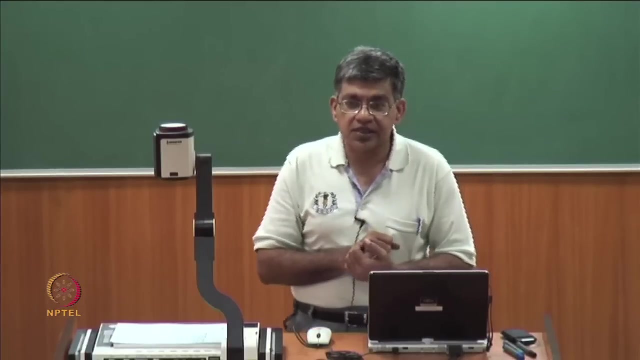 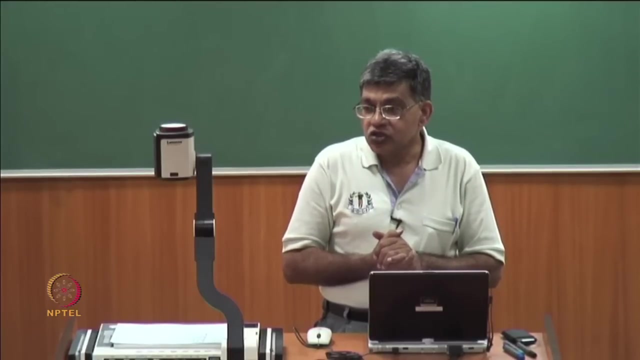 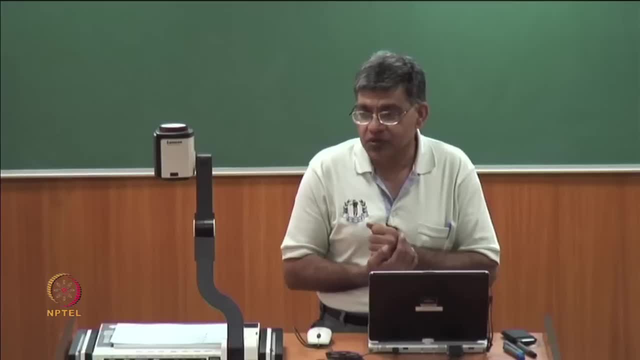 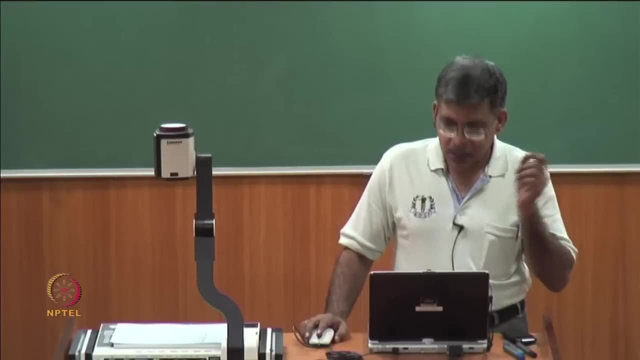 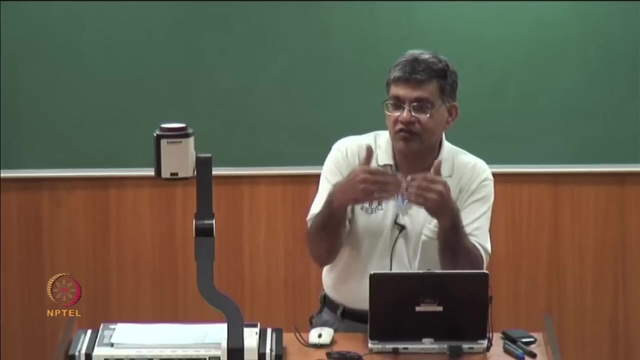 So that is a question that gets answered also by this Bahuban's theorem. So we will look at all these things, and so you can see that this notion of countable models is a direct extension of compactness, In the case of compactness. 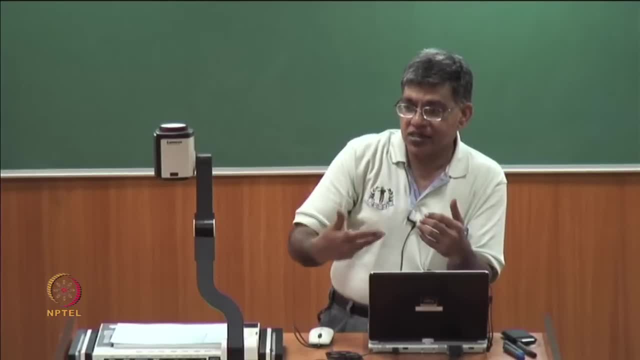 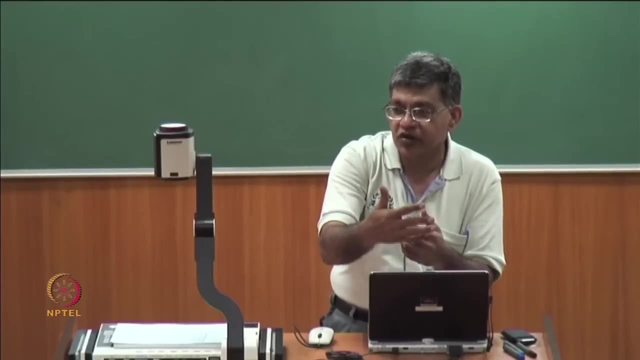 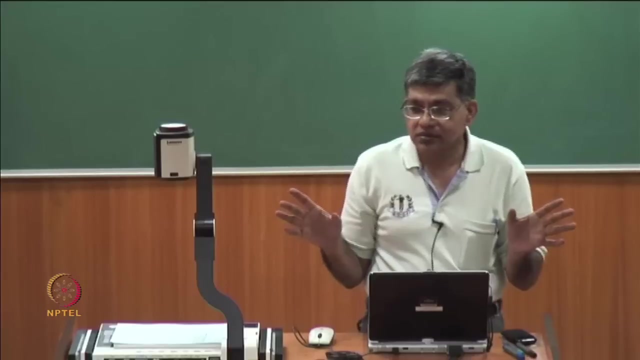 it was for a countable set, finite subsets Here, for even for uncountable models. you are saying that you do not need to look for uncountable models. you look for just countable models. that is sufficient. Finite models are not always guaranteed, but if every subset